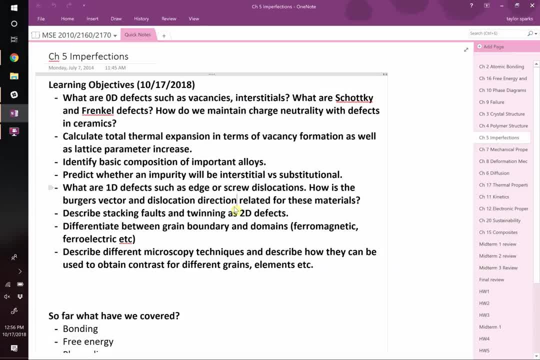 this Hector. what do you see? Yeah, it's rough. It's got kind of like freckles or little pock marks on it. so what's happening is that every time you take one of these ball bearings and drop it, you're denting the surface of that, because metals dent right, They're not the hardest. 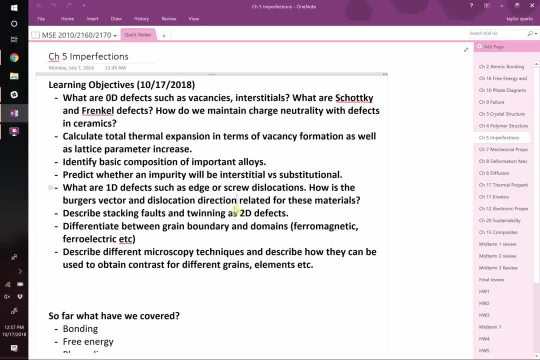 things. I mean some are harder than others, but they can be dented. and the reason they can be dented so easily is because you have a nice arrangement of atoms, right? If you look at sort of like the squares in this, right? if I was trying to slide atoms past each other because they're 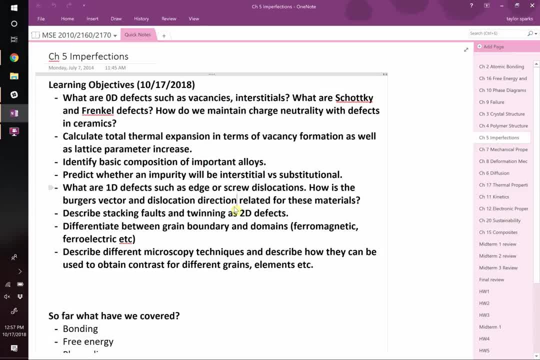 nice and arranged I could slide this row of atoms past the other ones, but if it was a jumble- and they're every which way as I tried to slide it- it's gonna bonk into another one, and so amorphous materials that. 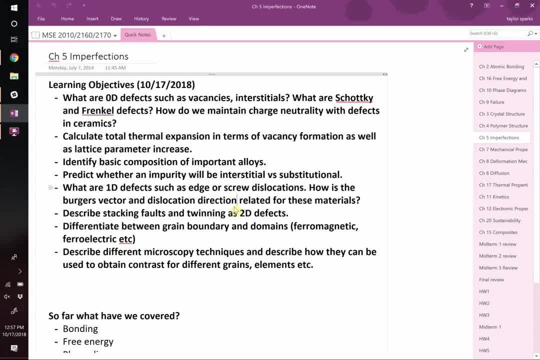 don't have structure tend to be much, much harder. and if they can't be dented, right, if you look at this one, it's basically mirror finish. It's much, much smoother than the other. If you can't dent the metal, then you can't absorb energy. If you don't absorb energy. 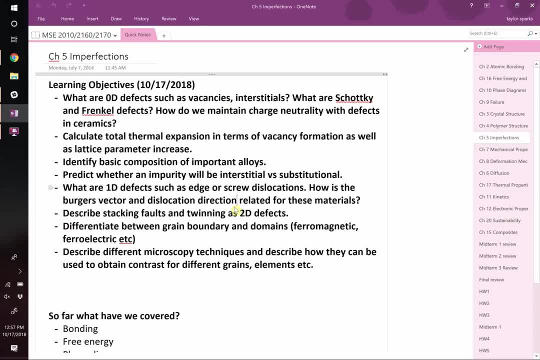 we don't just delete energy. It has to get transformed back into kinetic energy so it bounces back up high again, right? So that's a. it makes for a neat demo. but what could you use this for? Did we talk about that? 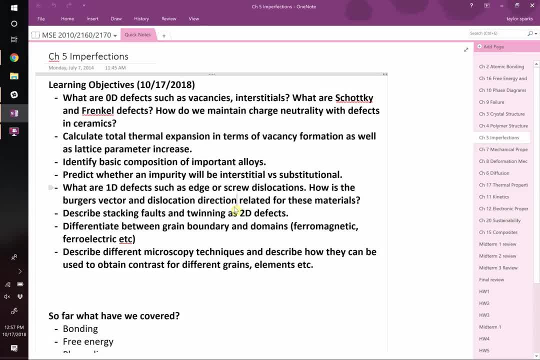 Did we talk about this? What would you use this for? Sport quirts? Sport quirts- How come You just want it to bounce better? Yeah, So actually bouncing is the reason they do this right and the application that I know of that exists. 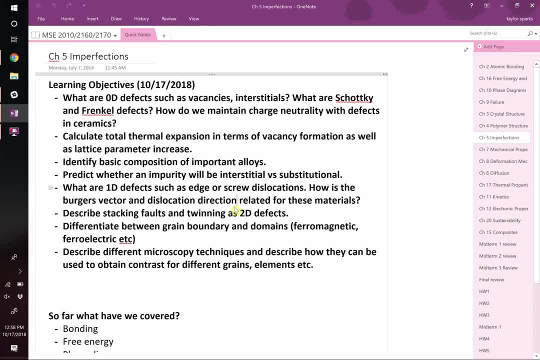 although I think it's illegal to use in some cases, is golf clubs right? So, if you're, I'm not a golfer, but like, apparently you want to hit this ball as far as you can, right, and so imagine what's happening. 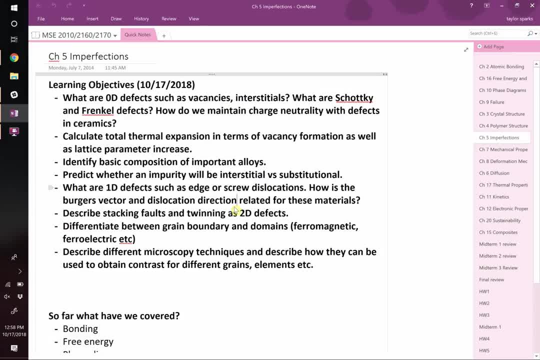 You've got your golf club and you're swinging it as hard as you can and you're smacking the ball, and then some of that energy is denting your club. Well, what if, instead of that, it just bounces further? right? 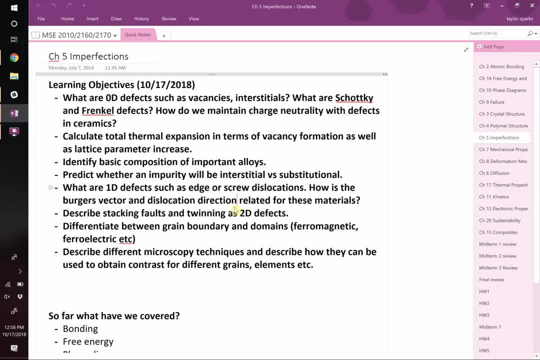 So you can actually make apparently tremendously good golf clubs Companies out there. they're called liquid metal. They don't make liquid metals, It's just amorphous metals. but there's- imagine there's- lots and lots of other applications. What if you just don't want something to scratch very easily, right? 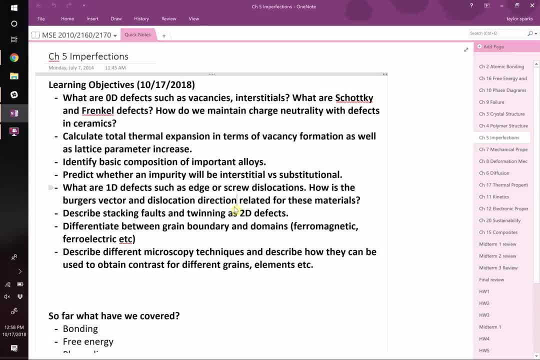 An amorphous metal is much more corrosion and scratch resistant, right, Anyway. so that's amorphous metals. The other thing that we're going to talk about more specifically today is a fuel cell car. right Now, this is like a toy fuel cell car. 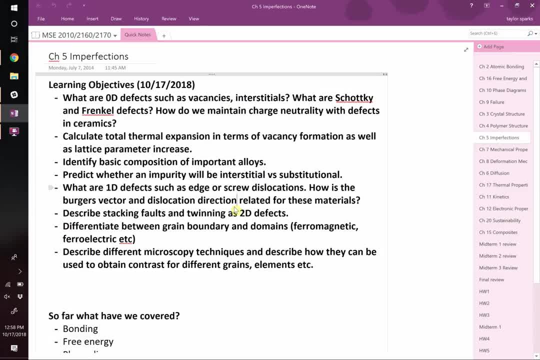 What goes into this is on this backside. you can pop this thing open and inside of it you've got a chamber where you put. sorry, you fill the bottom of this with water. okay, This is just a plastic container. and then it's got these little hoses that go through the cell. 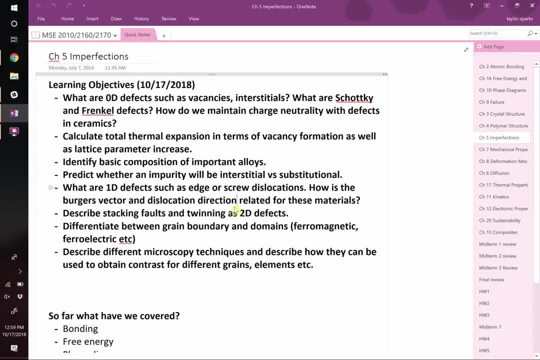 and then back into these gas chambers. So what you do is you start out by running this electrically, You provide an electric current and what happens is electrolysis of water. right, Electrolysis is splitting water into hydrogen and oxygen. That happens because inside, here in this middle piece, which is the size like an inch squared, 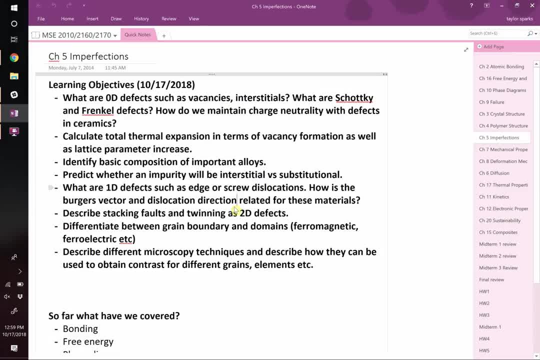 is a fuel cell. right, We'll describe what fuel cells are in today's class. Anyways, water goes in on one side. it splits it, it pulls an electron from the oxygen, sorry, from the hydrogen, making it H plus. 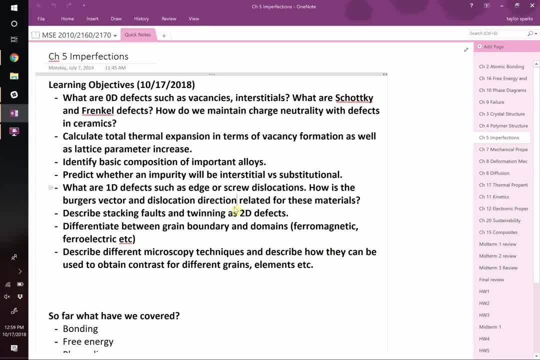 It takes and gives those electrons to the oxygens, making them two minus right, And now you have hydrogen and oxygen separated, And then, when you want to run this car, you disconnect the electricity, but now you have this reservoir of gases that you've created. 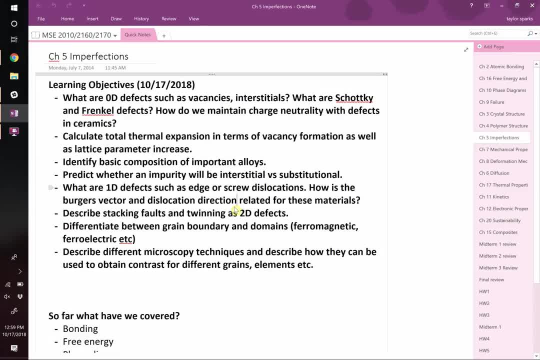 and they're going to recombine to form water. They're going to give off electrons which are used to power a small little DC motor here and you get an electric vehicle right. And this is a toy car, but the real ones exist right. So if you look, you can look this up right now like you could buy it today. The Toyota Mirai is a not terrible looking car that gets pretty remarkable gas mileage: 66, right, It costs a lot- 60 grand, but I don't know. 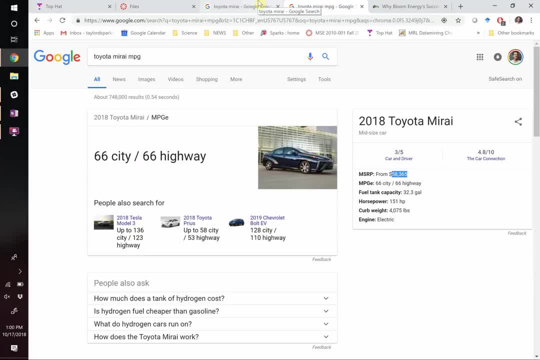 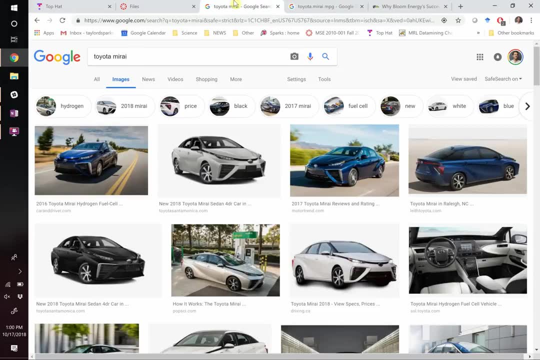 Nowadays you buy big trucks for 80 grand, right, Tesla Model 6s are what? probably 60k or thereabouts, or Model Ss I mean. So I mean it's not like it's a crazy price, but it's not the most economic price either. 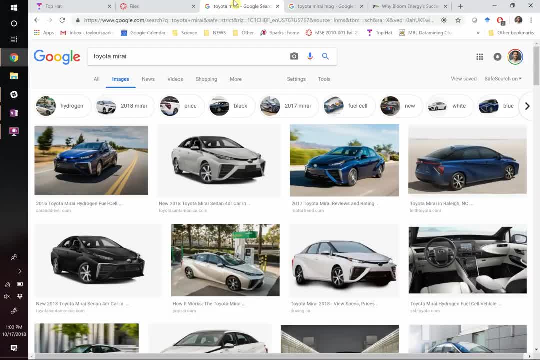 One of the great advantages to these over electric vehicles- which I'm a big fan of electric vehicles, but these have some advantages over them. The biggest one is that when you run out of gas, there is no gas in here, there's hydrogen right. 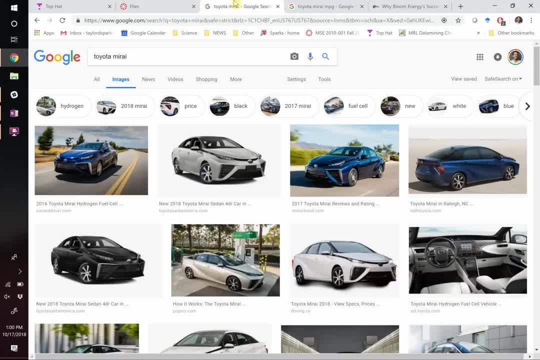 So you pull up to a tank right, a hydrogen tank- you refill and you're on your way in about the same amount of time as it would take to fill up gasoline in your car- possibly faster, right. So that's a big advantage. 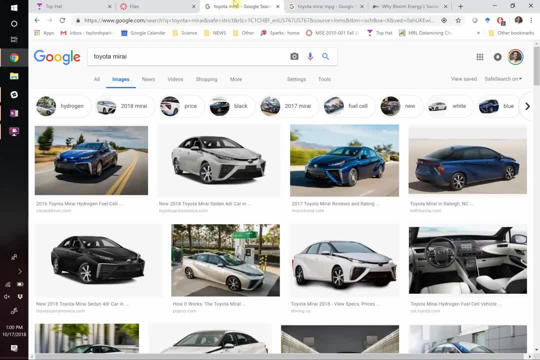 One of the disadvantages is what? What's the disadvantage to hydrogen cars Distribution? Sometimes people say like oh, these things explode, but like they've kind of got the exploding problem figured out right, Even if you crash, even if you crash one of these things. 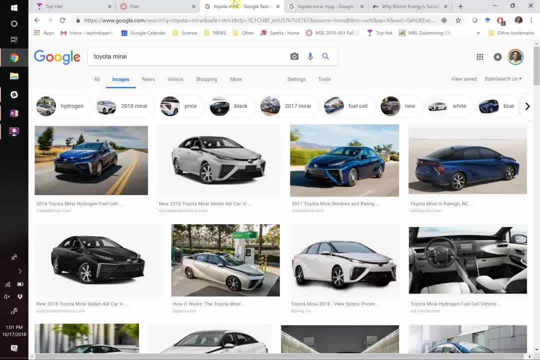 a friend of mine works at Volute, a company that makes the gas tanks for these, and they've actually tried to make these things explode catastrophically and it's hard to do. They use a carbon fiber serpentine coil, so it looks like your intestines right. 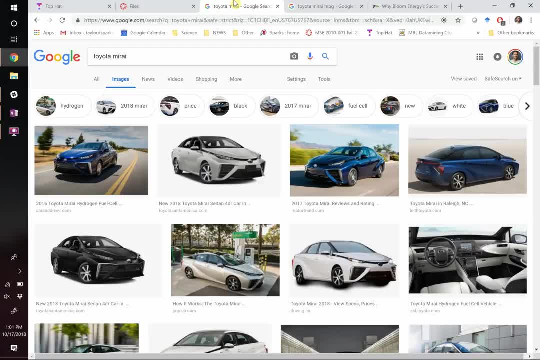 They hold the gas in something that looks like your intestines, but made of carbon fiber, and they've pretty well engineered this, so it's actually hard for it to explode. It's much, much more dangerous to crash a gas gasoline vehicle. 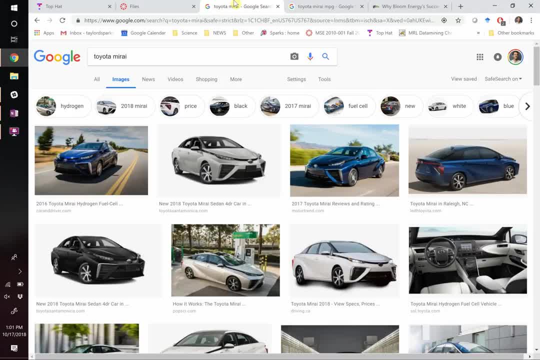 rather than a hydrogen vehicle. In any case, somebody up here said it, it's distribution. The problem with the Toyota Mirai is that if you buy it here in Salt Lake City- I don't know where- you fill it up with hydrogen right. 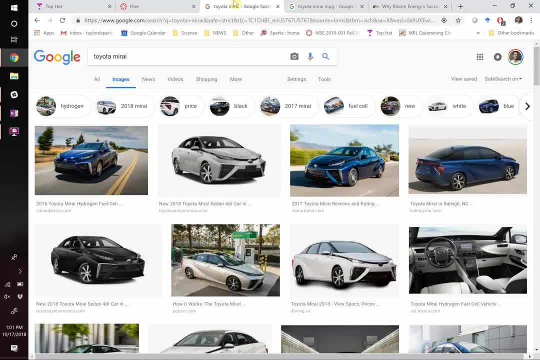 And there might be a place- I don't know of it So- and there's niche places in the Bay Area in LA, in New York City. there's sort of these beach heads where they've established fill-up stations, but for the rest of us it's not the most amazing option yet. 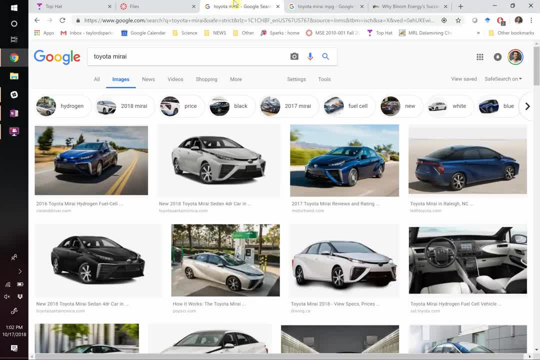 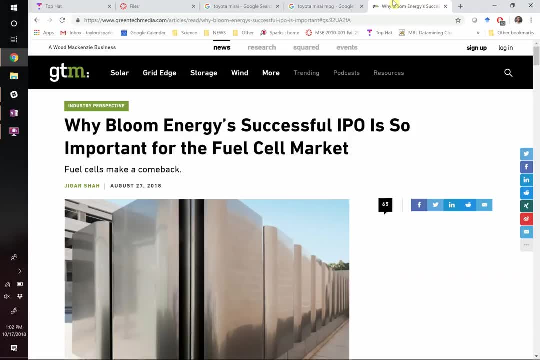 because of infrastructure, right. So hydrogen is not just important for vehicles, right. It's very important for energy, right. A couple of months ago- this was in August, right. Fuel cells have been around since the 70s. 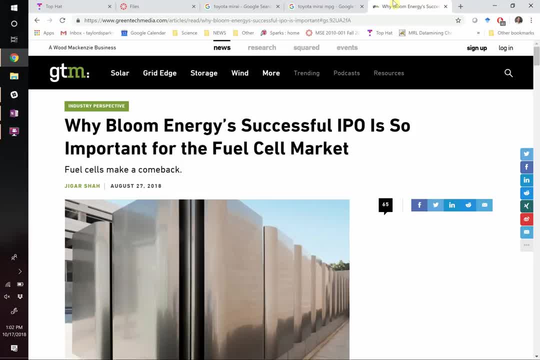 but they're making a pretty big comeback. One of the biggest companies in the energy sector did a big IPO. It was like a quarter billion dollar IPO. It's a big public offering And essentially they're banking on these for renewable energy storage. 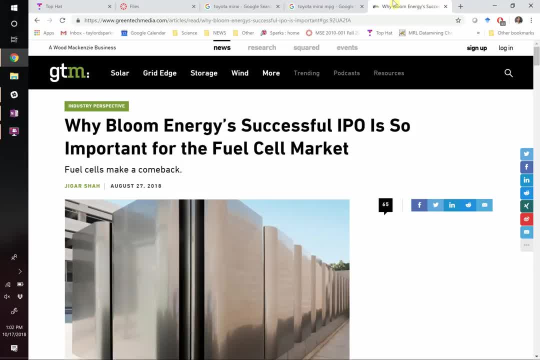 So let's say we all believe in renewable energy. The big question is: you know, what do you do to provide energy to people who need it, when the sun's not shining or when the wind's not blowing right? These are the challenges that we face in renewable energy. 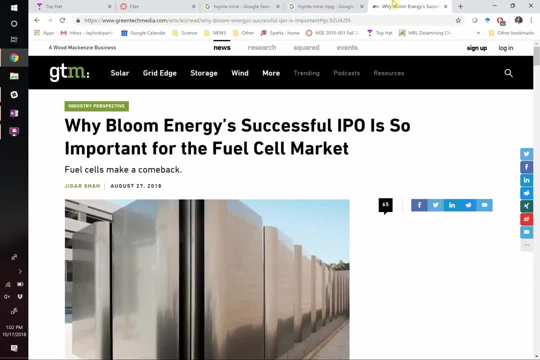 You have to have a way to store it, and one of the well, the cheapest way to store it is what? What's the cheapest way to store energy? Anybody? It's surprising what they do. It's pumped hydro. You take a reservoir of water. 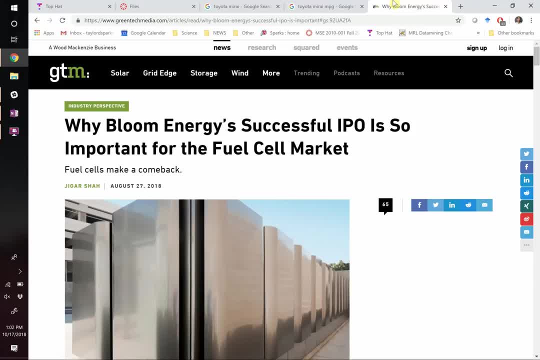 and you pump it up to a higher reservoir with the electricity you're generating, right From solar or whatever- And then, when you want to get that energy back, you run it back down through the hydroelectric mill. right, You can do that on a small scale, like a water tank in a small town. Or if you live by a mountainous area and you've got a dam up in the mountains, you can pump it up into the reservoir up in the mountains. That is the cheapest way to store electricity right. Currently it's pumped hydro. But that only works if you have a place where you can store lots of water right, And that's not the easiest. plus, it has its own challenges with it. So if you don't want to do that, one of the most promising areas that's coming online is fuel cells. 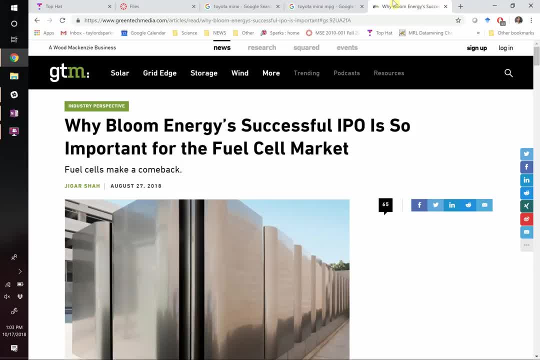 There's batteries. You could put it in batteries, or you could do fuel cells And a fuel cell, just like I showed you. you could take electricity right, Just like this car did, like a 9-volt battery or a little solar panel that it comes with. 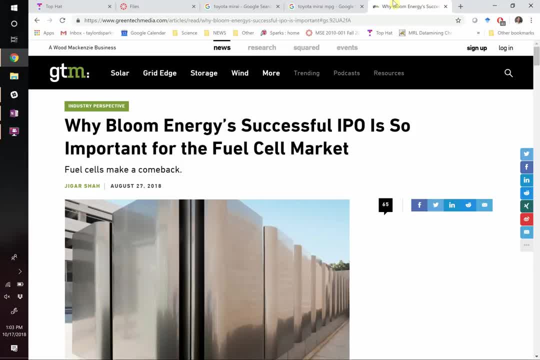 You could take that energy and you could split water into those two gases and then recombine them at your leisure whenever you want right? That's the idea behind these, So fuel cells. the whole point of explaining this is that 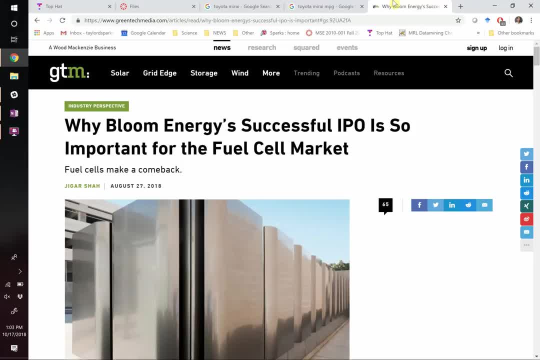 they would not function if it weren't for imperfections in a material. A perfect fuel cell is a perfect material, where every atom is in its place, where it's a perfect alloy right, All just a certain type of atom, They would not function. 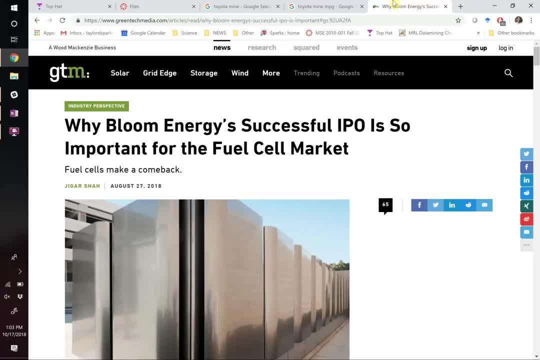 And we're going to describe today why. Why is that the case? okay, And by the way, fuel cells look something like this: Like this is a stack. I don't know what power this is. This is probably like I don't know what power this is. 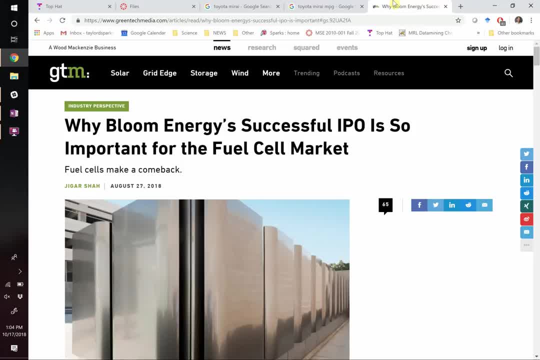 But they're layers of ceramic membranes. They don't have to be ceramic. There's polymer ones too that are put together and you essentially have, like your air in and your fuel gas coming out, and then this would be hooked up to electrical leads. 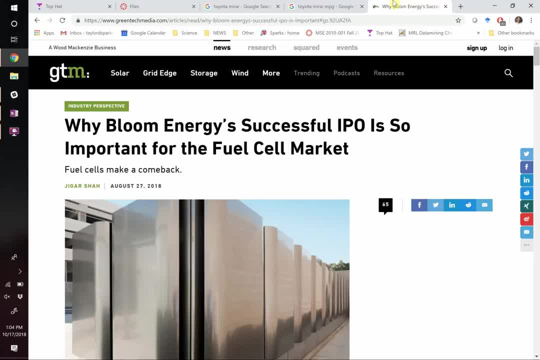 and you generate your power. So they're small. These things aren't gigantic. They're small And there's sort of there's advantages and disadvantages to the fuel cells. We won't get into them in this class because it's not specifically on energy. 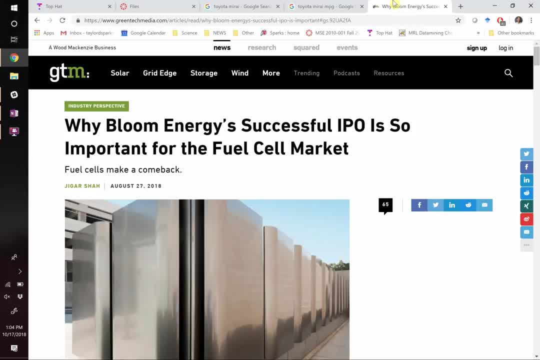 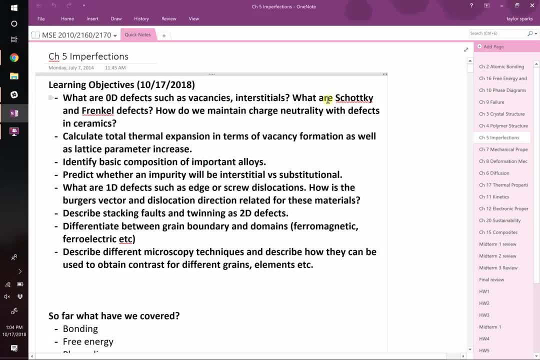 But I think it's a technology you should be broadly aware of. Okay, All right, So let's dive into today. We will talk about the things we talked about last time- The same objectives, because we didn't get very far. 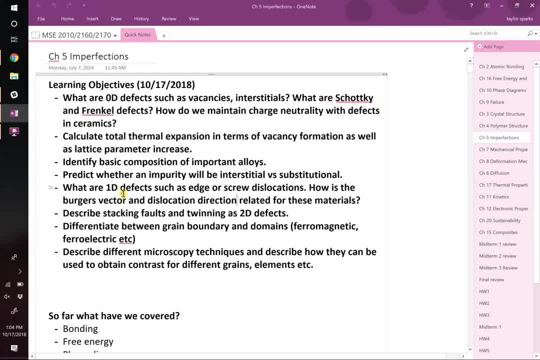 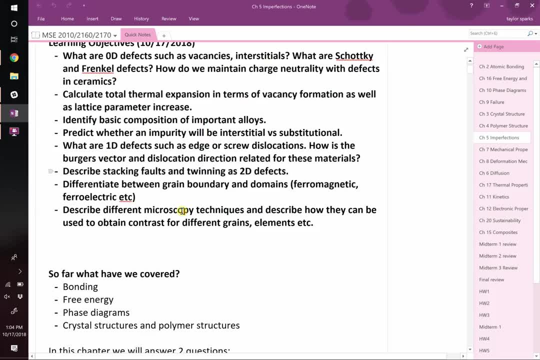 And, if possible, we're also going to move into one-dimensional defects. So we're not just going to talk about 0-D point defects, We're going to talk about one-dimensional defects in materials. okay, And we'll see how much further we get. 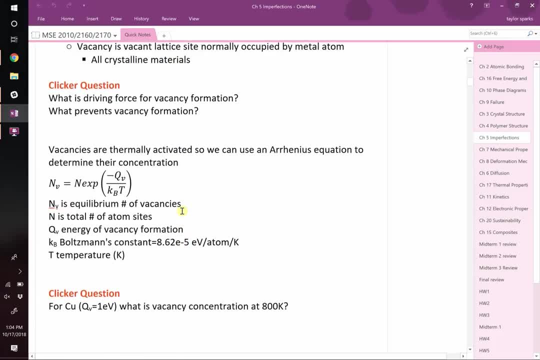 So we can see we talked about the driving force for vacancy formation and the one preventing it. We said entropy is typically driving it And enthalpy, or breaking these bonds, is preventing it. Actually, Avery, I'm sorry. 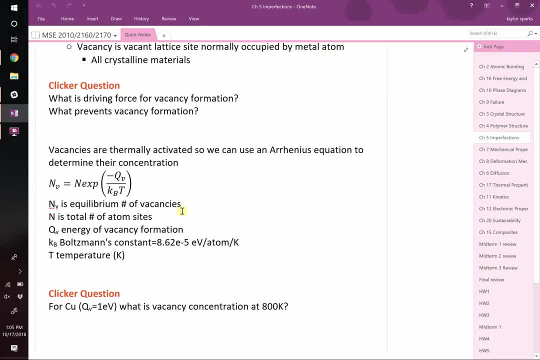 I forgot. Do you want to talk about the Bennion center, Or do you want to wait until the end of class? Stop me when we've got five minutes at the end of class. Okay, So vacancies. How do we know how many there are? 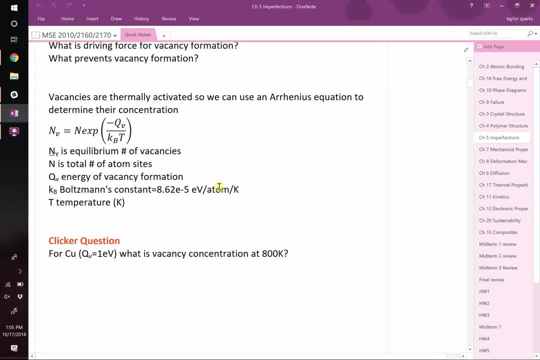 in a given material, We use our old friend, the Arrhenius equation, Remember. the Arrhenius equation is when any property of interest, like Nv, the number of units or the number of vacancies- at equilibrium if it depends on something. 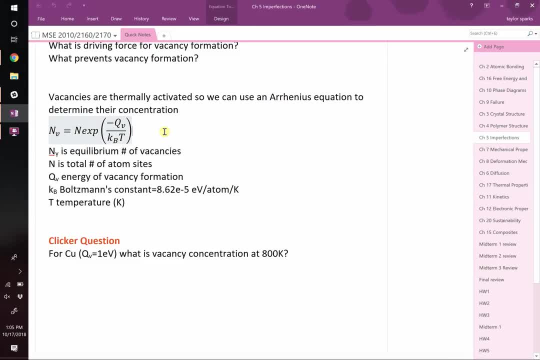 where there's an exponential with an activation energy, in this case q sub v. that's the activation energy for vacancy formation divided by the thermal energy: kbt, Boltzmann, constant times, temperature. that's an Arrhenius type of equation. 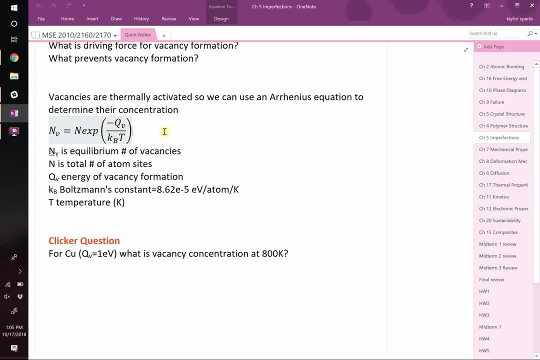 So we can figure out the number of vacancies at any temperature. if you know the following: N, that's the total number of sites, right? So in a crystal lattice, right, Let's say FCC for a minute In FCC. 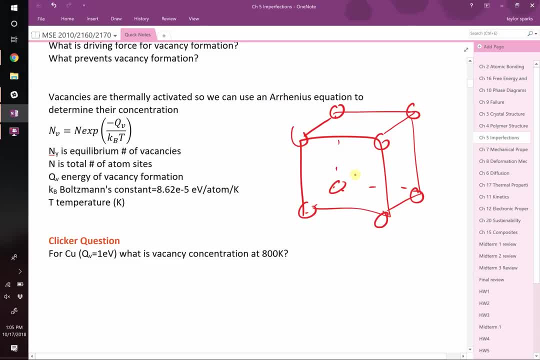 you've got these atoms right, That's on the corners. then you've got front, back, top, bottom, left, right. So you can figure out what the site density is. That means how many sites are there per volume? 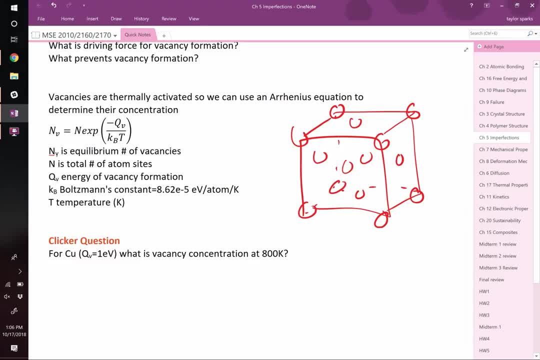 And we know that there's four sites, right, Because there's four atoms in this crystal structure. There's four atom sites per some volume, right? So that would be N, That's your site density, And then Mc we calculate once we know. 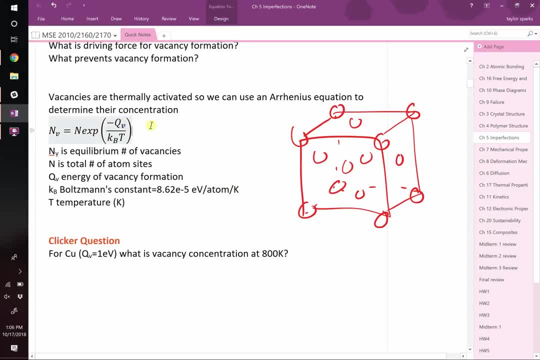 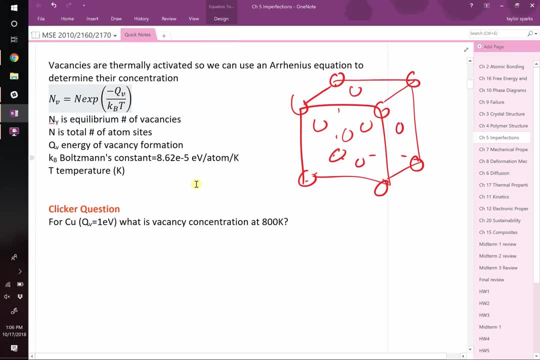 the activation energy for vacancy formation. So let's go ahead and do a quick example of this. This will be our first clicker question. We're going to do it for copper. Copper has a vacancy formation energy or an activation energy for vacancies. 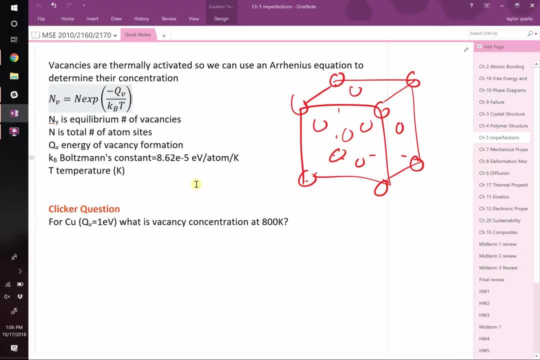 of one electron volt. So I want you to tell me what would be the vacancy concentration. Concentration is going to be Nv divided by N, So you're just going to bring N over to the left-hand side of the equation at 800 Kelvin. 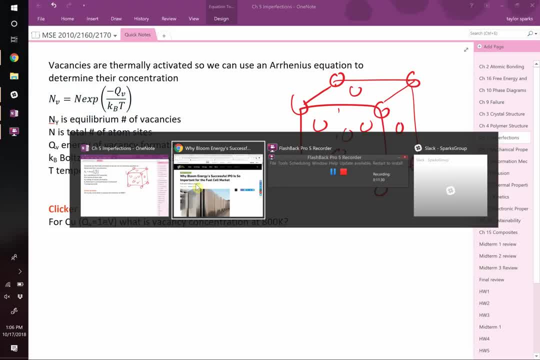 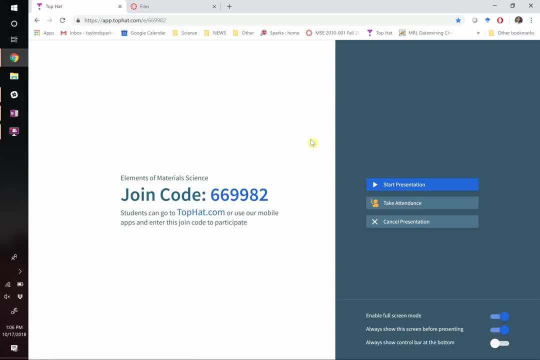 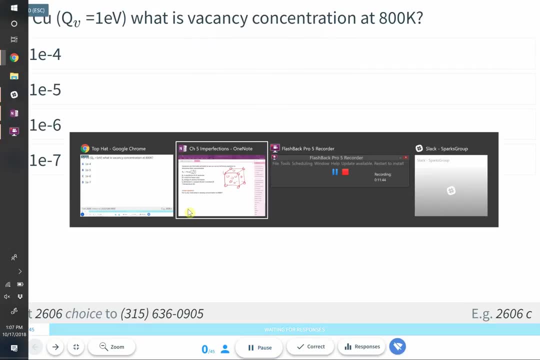 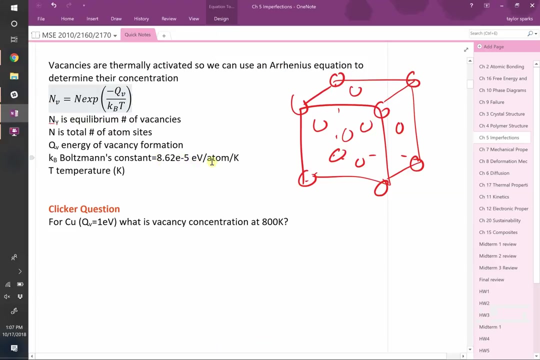 So give that a shot. We're going to pull it up on top hat And K. right there, your Boltzmann constant in electron volts is what you want. That's going to make this a more convenient calculation, since the activation energy is given in electron volts. 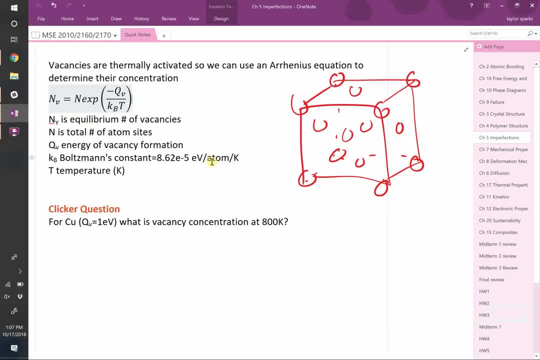 not kilojoules per mole or something. There's Kb with electron volts per atom per degree K. Okay, we'll do one more minute. What's up? Tell me one of those works. You're searching for Nv over N, right? 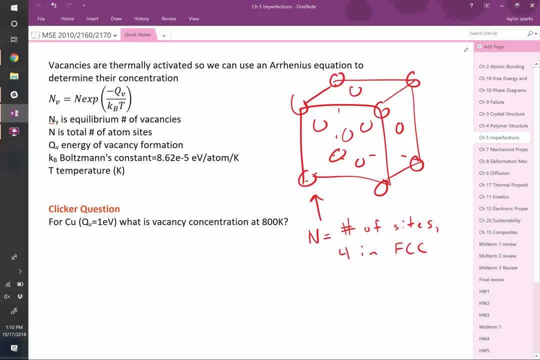 Yeah, Nv over N is what you want. Yeah, So all you have to do is plug in the exponential. Yeah, plug it in, but it's not one of these. Oh gosh, It's like the same magnitude. 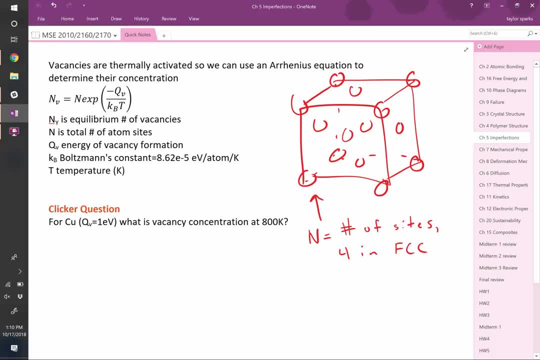 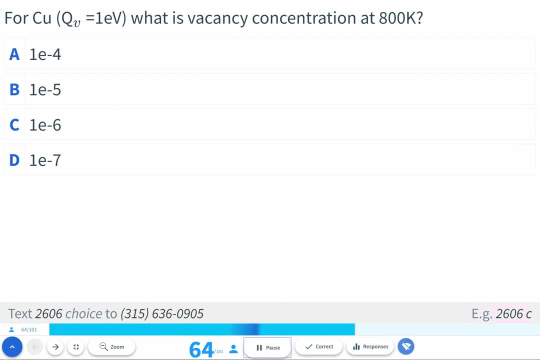 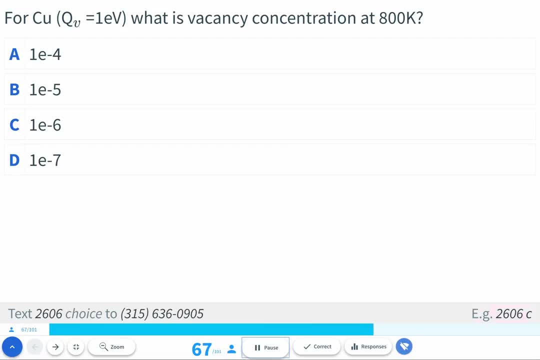 is not one of these ones, Pick the one that's closest to it. The right order of magnitude. I'll double check my calculation. Maybe I messed up on this, But Okay, just we're going to wrap this up pretty quick here. 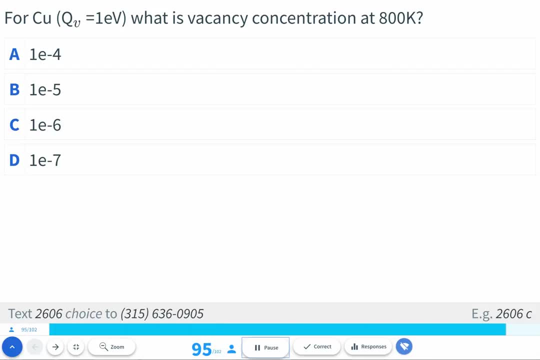 What's that? yeah, I'll double check after class. okay, we're going to close the poll. okay, and people think this should be, oh interesting. alright, I will find out what went wrong. I'll probably give you credit for either of those, because I don't think it was bang on one of those numbers. 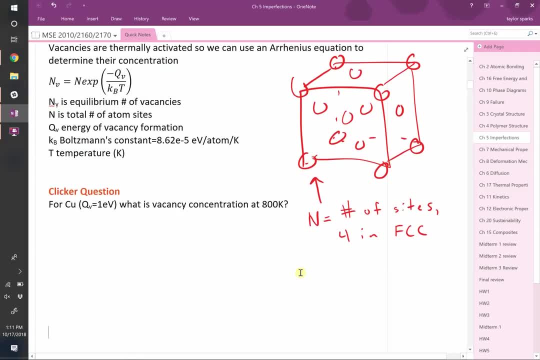 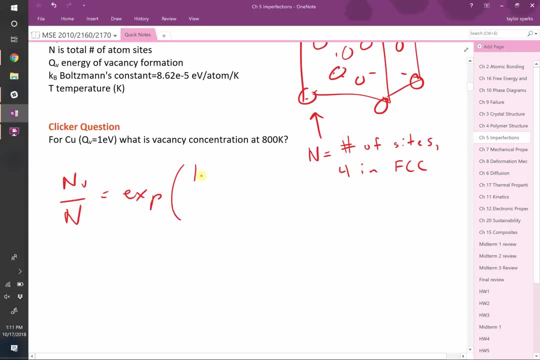 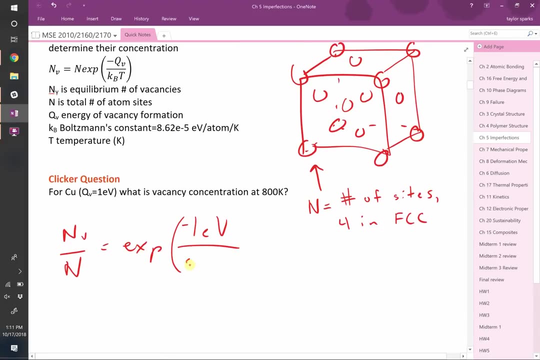 so how do you do this? though it's a straight forward calculation, let's do it together: nv over n is equal to the exponential of one electron volt. that's negative one electron volt because it's negative q. right negative q divided by this is 8.62. 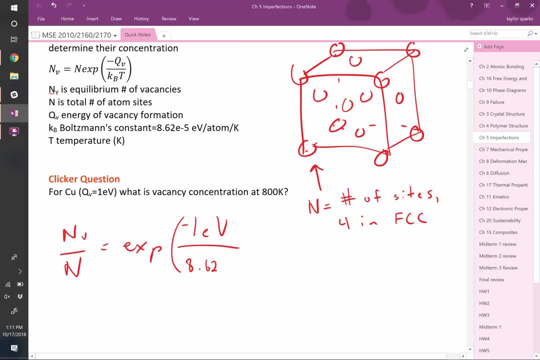 I wonder if that's the actual value, I wonder if it's a rounding issue. but anyways, that's times 10 to the negative 5, that's ev per k, and this is all happening at 800k. so when I plug those in, I get, I get. 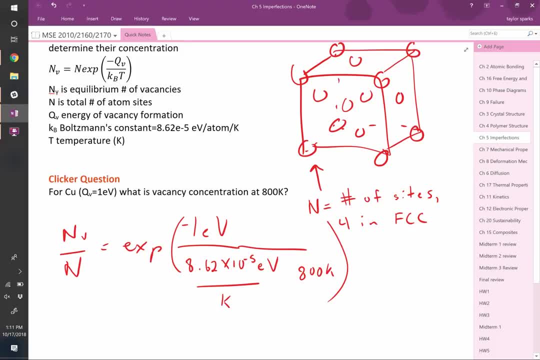 5e to the negative 7. anybody else get that? 5e to the negative 7 and again. so what would the units of that be? what would the units of this be? so it's number, it's the equilibrium number of vacancies divided by the number of sites. so that has. 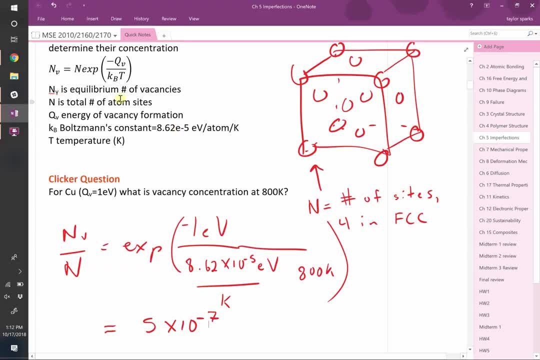 no units, right? this would be like saying percentage, right? you could put this in parts, per million, if you wanted, you could, but it's just a, it's a fraction right now. okay, any questions on this type of question, on this type of problem? yeah, so nv over n is. 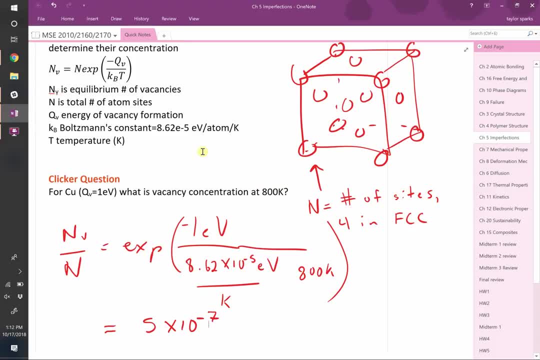 the concentration we're trying to solve. so I guess I asked for vacancy concentration, right? so yeah, technically, if I said what's the vacancy concentration, like the number per volume, then I'd have to tell you things like what's the lattice parameter, because in that case- and you're going to have a homework question- 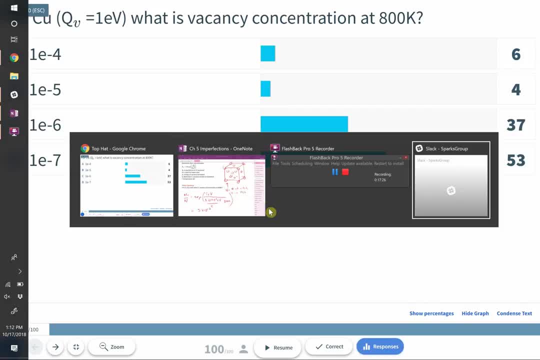 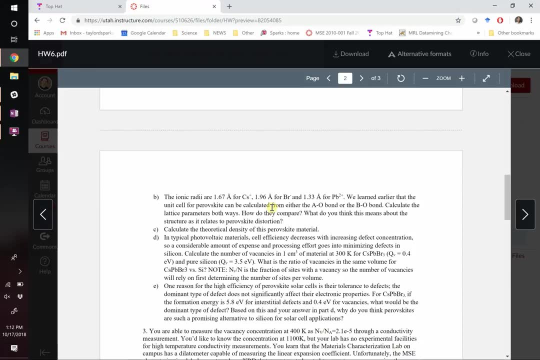 on that. by the way, quick announcement on that: the homework is posted. let me pull this up real quick. the homework is posted, but I had to change one thing, so if you downloaded it like the second that I posted it, make sure that you got the right copy. 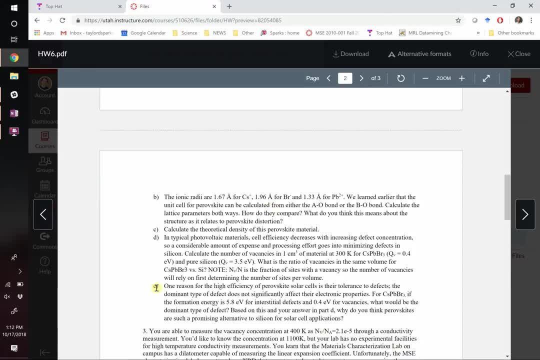 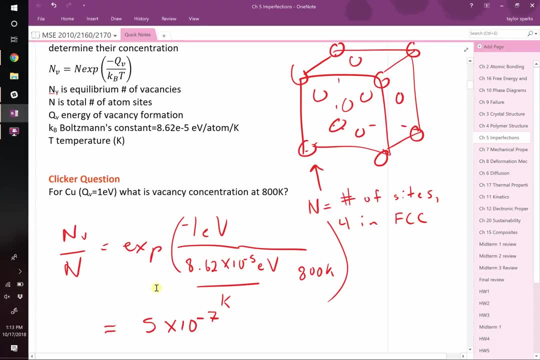 problem 2 should have parts a through e. if it doesn't, then you download it too quickly. but on the homework you're going to have an example where you have to download, you have to figure out the number of vacancies per volume and in that case you need to figure out. 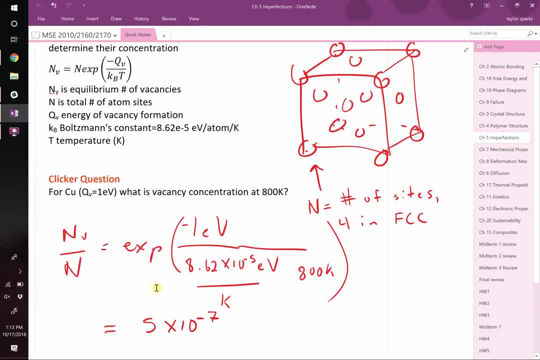 nv right the number of sites and you need to figure out how many sites there are per volume. that's how you do it, how you'd get the number of vacancies per volume. So you have an example to do that on a homework And I think I've got YouTube videos where I've 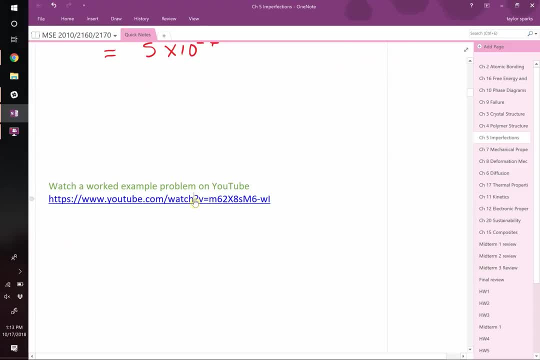 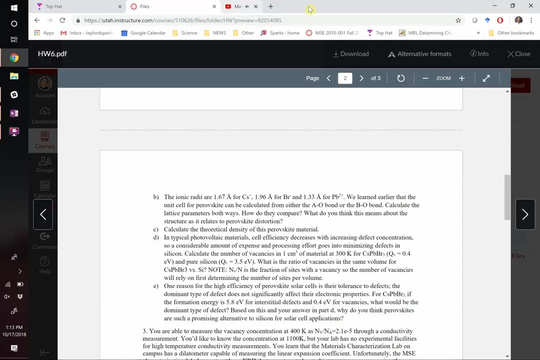 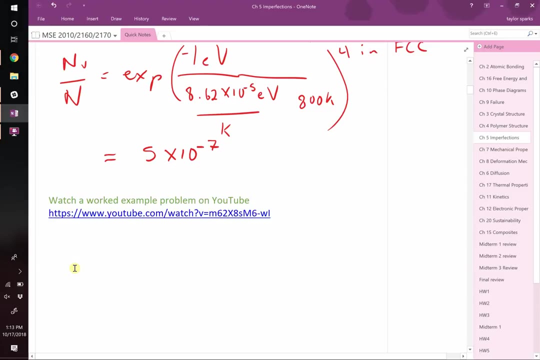 worked through that as well. solution videos: This is probably one right here. So here's an example where you can go through the same sort of calculation. Any questions on this? On vacancy formation: So if you compared two materials and all things equal. 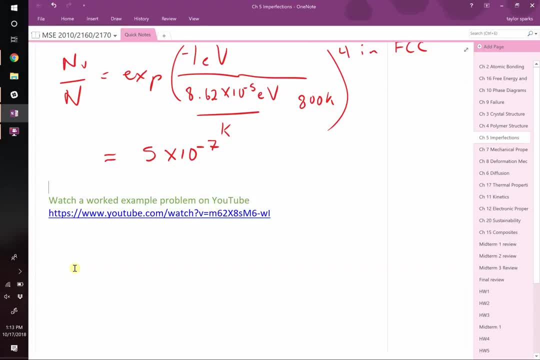 if they've got the same number of sites per volume. let's say they're both FCC, they're both similar lattice parameters, but one has a gigantic activation energy and one has a really small one. you know, the one that has the small activation energy. 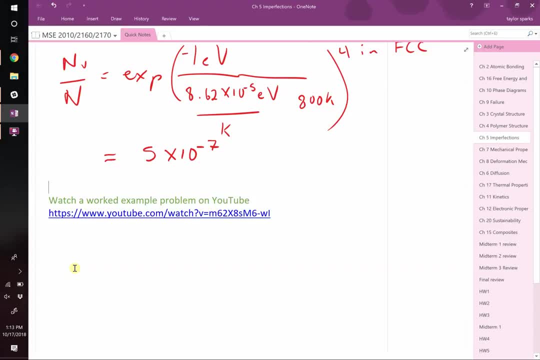 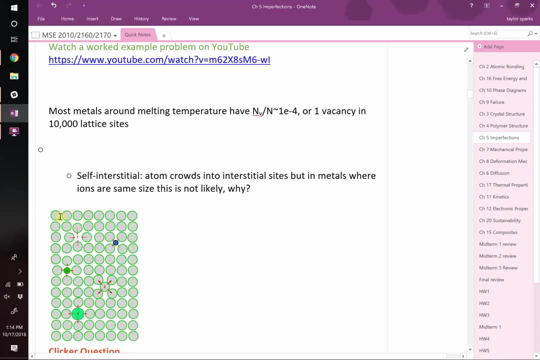 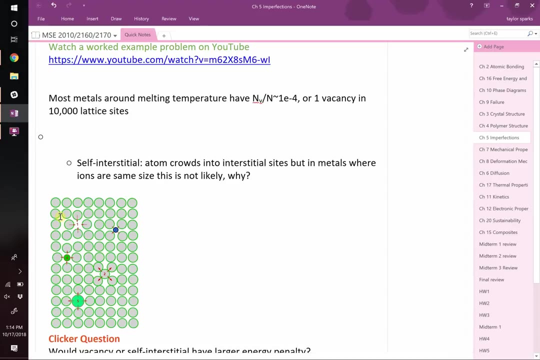 is going to have way more vacancies than one that has the really big activation energy. So how much are we actually talking about? How many vacancies can we even get in materials? So take metals Even at their melting temperature where you've heated it up about as much as you can heat it up. 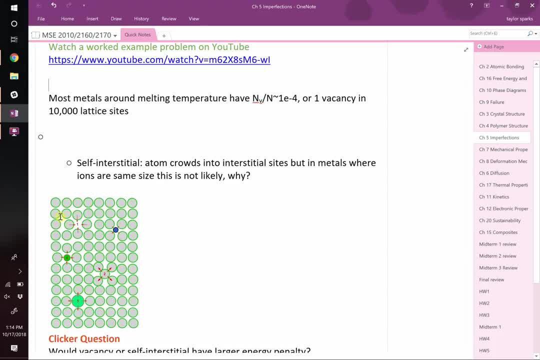 right Where you're right there before it becomes a liquid and vacancies don't really have the same meaning anymore. Even at that point, most metals have nv divided by n of about 1e to the negative 4, which means you have about one vacancy for every 10,000. 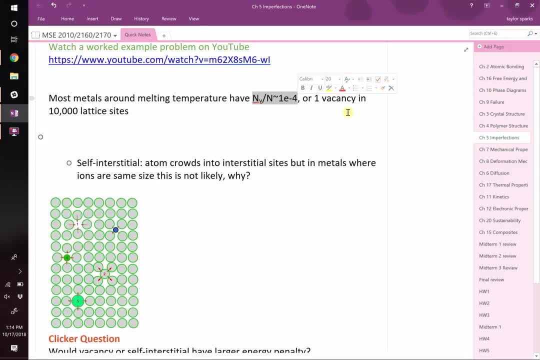 lattices. So these things are not like everywhere typically right. The vast majority of compounds. they're not like riddled with vacancies, They're pretty rare. But even at the 1e to the negative 4 amount they can dominate properties. 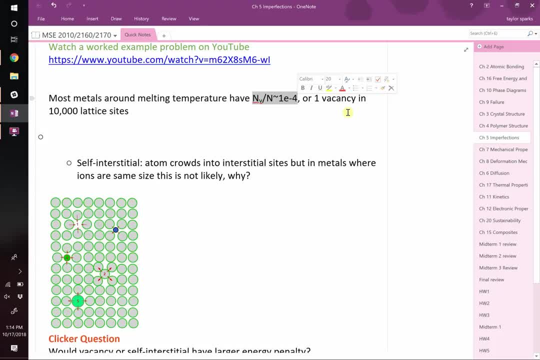 They can really influence properties- Some of those we have We haven't talked about in this class yet. like electronic properties, They are very important to how electrons travel through a material. They can be dominated by vacancies, right, And that's going to be the case in fuel cells, OK. 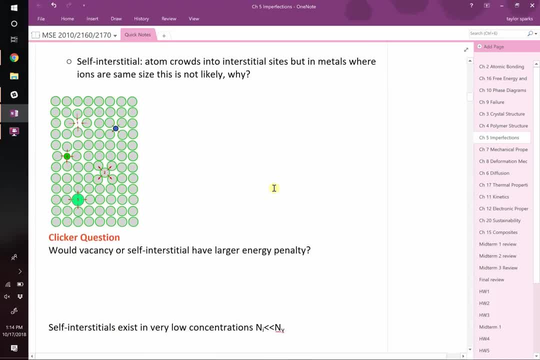 OK, there's other types of defects we can have. There's vacancies and then there's self-interstitials. is the other one point defect we'll talk about. So a self-interstitial, let's say, you had an atom like this gray one at point number 2 here, right? 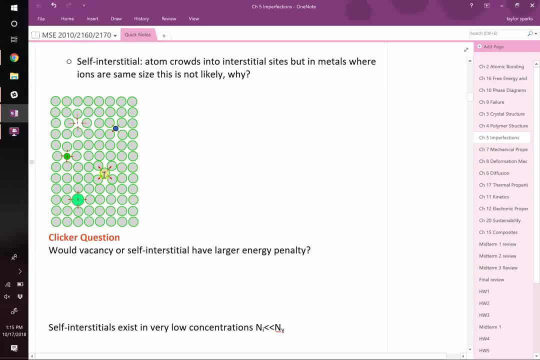 You can see that you have a lattice of gray atoms, But here somebody's crammed in an x. It's an extra lattice, atom number 2, which we call- point sorry- gray atom, which they call point 2. on this, OK. 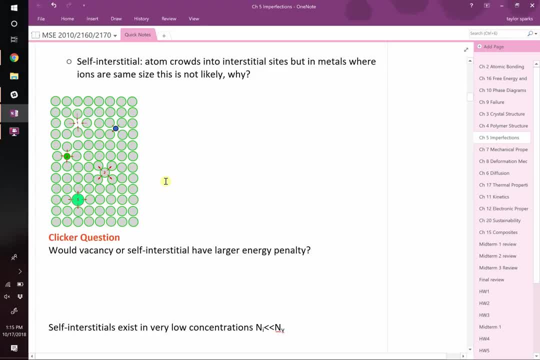 That's an example of a self-interstitial. Generally speaking, is this my next clicker question? Oh, right, here. yeah, Would vacancy or self-interstitials have a larger energy penalty? right, So it's our next clicker question. 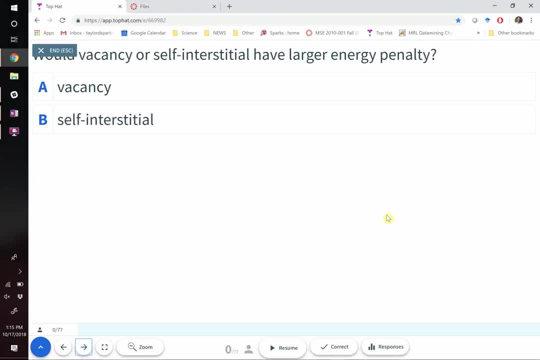 If you read the text, you should know this: Which one of these comes with a larger energy penalty? Is it the vacancy, Or is it the, The self-interstitial? And if you're struggling on this one and you're not sure, 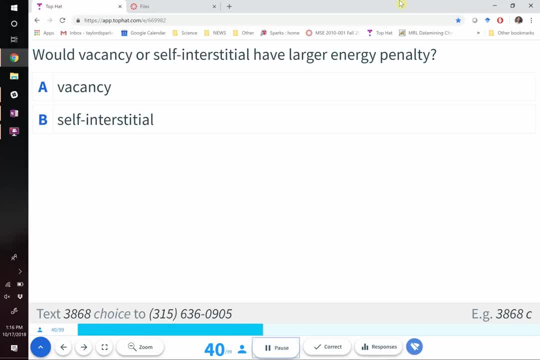 ask yourself which would be a more awkward situation If you had a bunch of people lined up nicely and you took one out or you put in like an elephant in the room. like which one's more awkward? OK, we're going to close the poll. 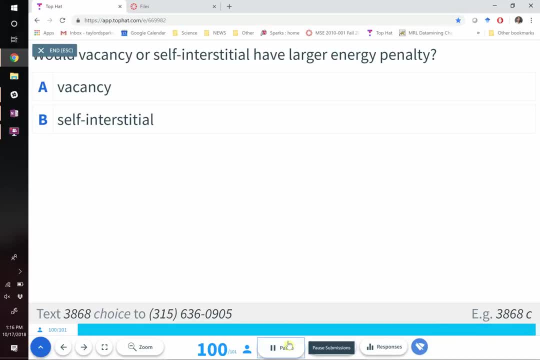 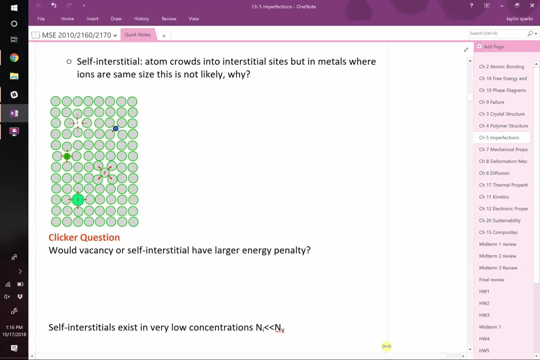 OK, good Man, this is just always the case. It's always like 15% of people are getting these wrong. Sorry, But interstitials cost more. They have a larger energy penalty, and the reason why is because they strain the surrounding. 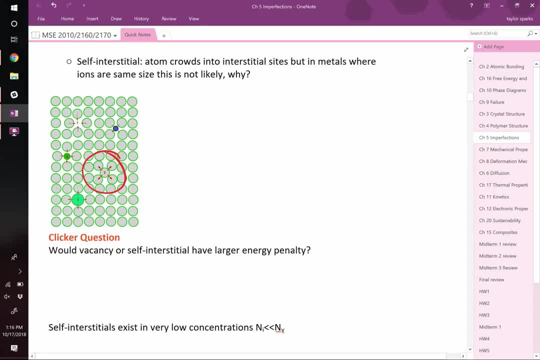 lattice a little bit more. If you look at this, if you zoom in on that, it's not just the one spot that's messed up, but the nearest neighbors. Look at these, These nearest neighbors. they're also pushed out of position and so forth. 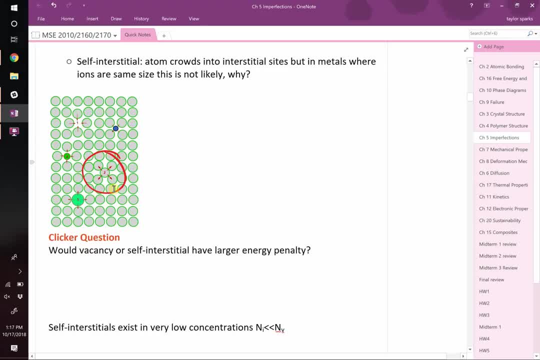 It has this ripple effect on the surrounding atoms, which is going to compress bonds that don't want to be compressed, In general compressing things if we go back to our potential energy. well, which we will go back to over and over and over in this class, as you separate atoms, they have their 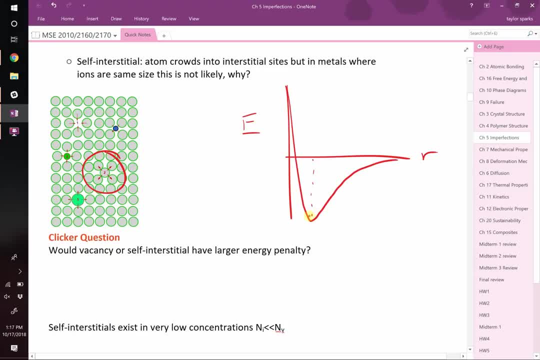 equilibrium distance and then they tend to be steeper. on this side That tends to be a little bit sharper and a little bit less steep over here. So if you're squeezing things together you pay a big energy penalty for it. So when you have a vacancy they expand a little bit, right. 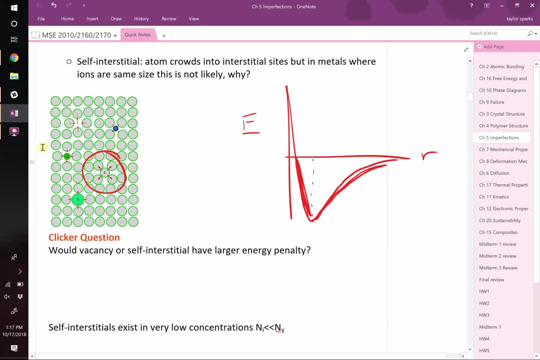 Look up here at point number one. In that case the atoms are sort of pushed out a little bit from their normal position. but that is less steep, right, It's less of an energy penalty In general. cramming something into a lattice is a much higher energy penalty okay. 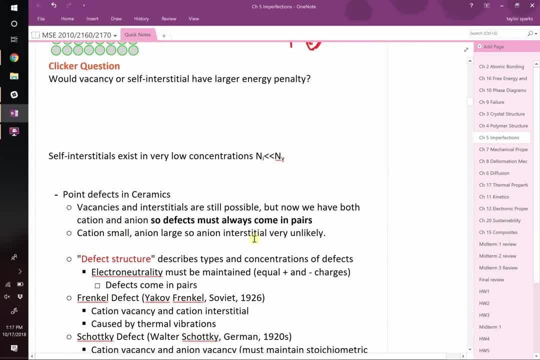 But that's self-interstitials, right. So again, self-interstitial means you have a copper lattice and the extra copper atom that's out of place is a copper atom, right? It doesn't have to be the case that it's a self-interstitial. 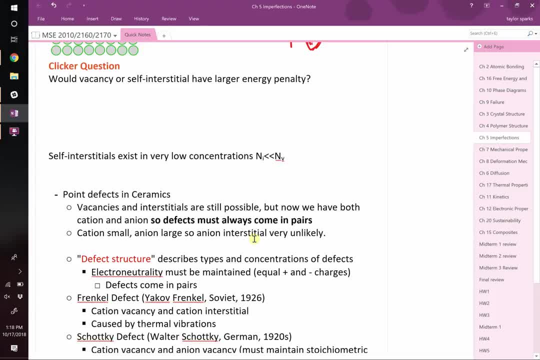 You can have other things. You can have dopants. Let's say you have a copper lattice and you put a nickel atom in it. We know that there's a solid solubility all the way across from copper to nickel, but they're not the same size. 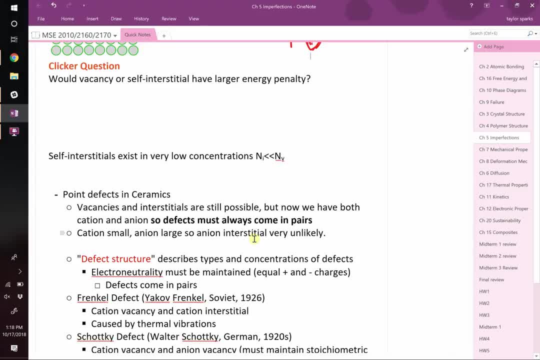 They don't have exactly the same capacity, They don't have the same chemical characteristics, and so there will be a chemical penalty, whether it substitutes, meaning it sits on the site, or it goes interstitially right. All right. So let's talk about point defects in ceramics. 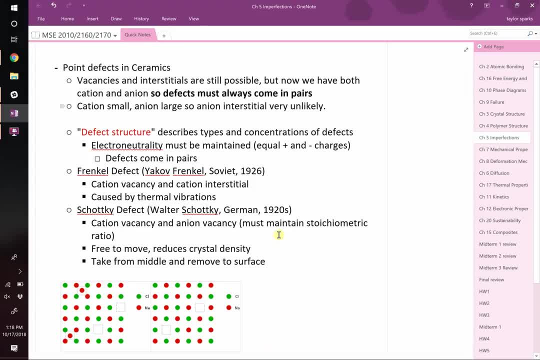 In metals it was straightforward: You have vacancies or you have self-interstitials or about all you have. In ceramics it's harder for the same reason that crystal structures were harder, because there's different sizes and there's different charges on them. 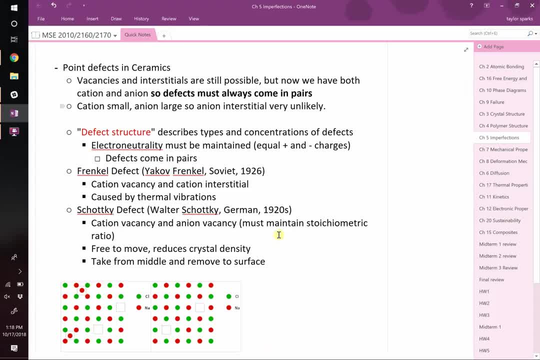 That leads to the same problems here with point defects right. The different charges and sizes leads to defect structures forming right. And there's two important ones we have to know about. There's Frenkel defect, named after Yakov Frenkel, a Soviet in the 20s, and Schottky. 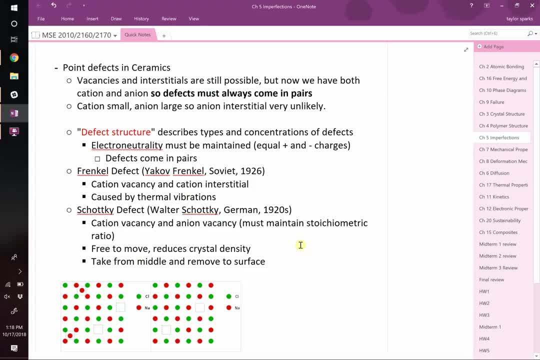 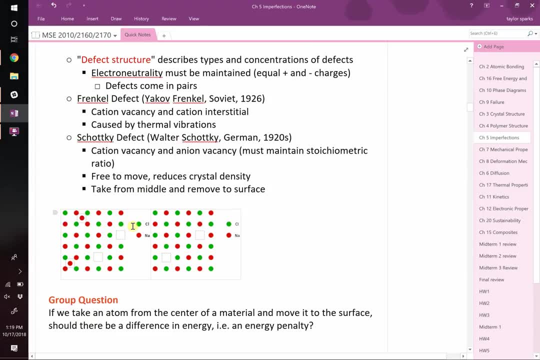 defect named after Walker Schottky, a German in the 20s right. So here's the difference A Frenkel defect is when you take. Let's see Which one's which down here, Let's show you. 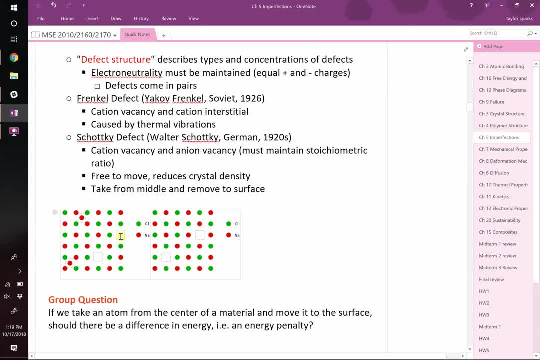 A Frenkel defect is when you take it out of its normal site, like this empty spot here. That should be a red atom, Right, It's missing. This one should be a red atom, but it's missing, right? Those red atoms are located elsewhere in the structure, right? 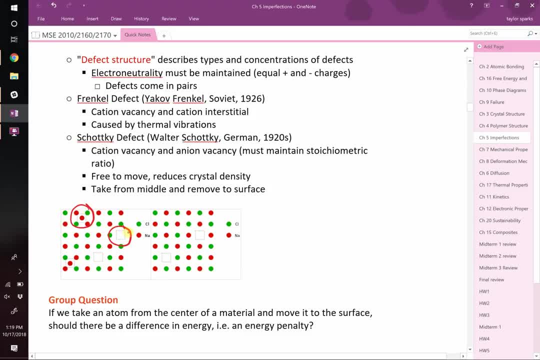 You see that. So they come in pairs. This thing left and now it lives somewhere else, So it's a pair. You have both a vacancy and an interstitial. That's called a Frenkel defect. A Schottky defect is different. 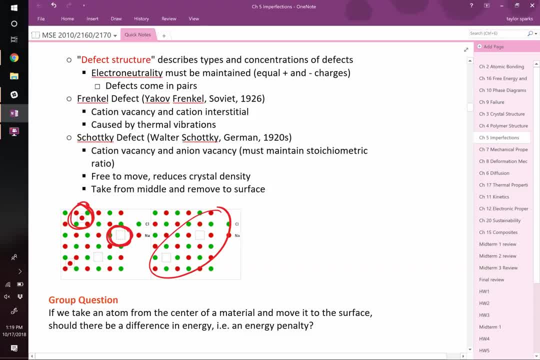 A Schottky defect is like this one: You have two vacancies, one of each type. So in this case it was a red atom that was missing, But that red atom was just located somewhere else. In a Schottky defect, you're missing a red atom and you're missing a green atom. 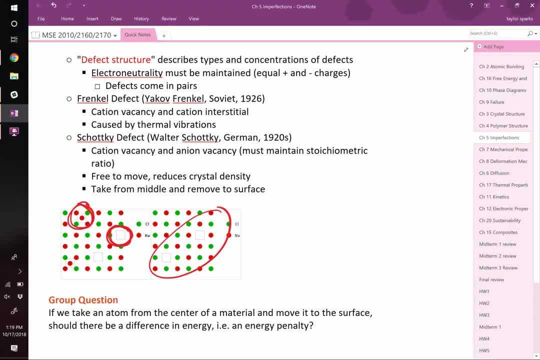 So use whatever mnemonic device you have to come up with. Here's mine. Frenkel sounds kind of like a creepy name. Sorry to the Franks in the room, But Frank sounds like a guy who doesn't respect your personal space, Right. 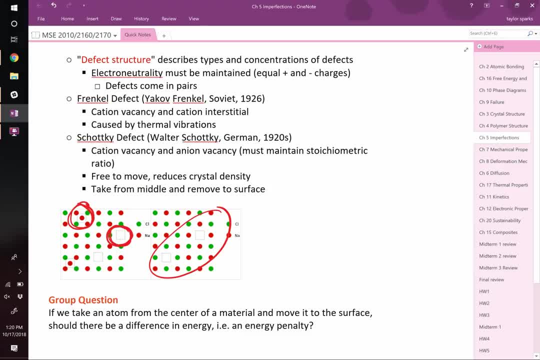 Come on, Frank, He's not respecting personal space over here, But, Schottky, it's like he shot a hole through it. They're both just missing. So that's what I use. Remember it, however you will. But those are the two most common types of defects in ceramics. 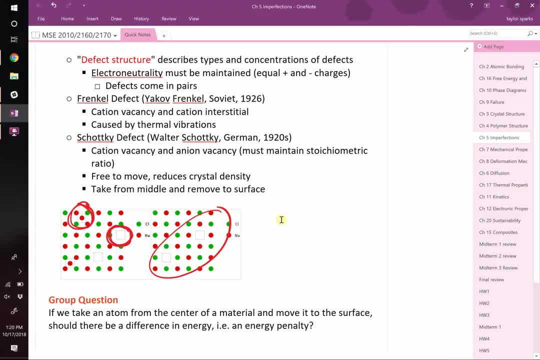 There's tons of others, right, And these are for pure materials. right now. We haven't even doped these yet, right? This is just like say it's sodium chloride. These are defects that can exist in the pure NaCl. 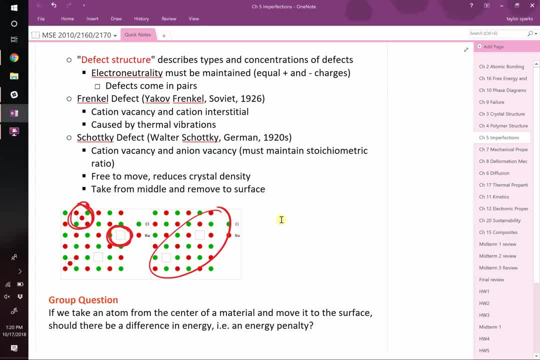 What happens if we start doping sodium chloride with something else? We put a little bit of calcium, which is now two plus right? What's that going to do? Sodium is one plus. You put in a two plus ion. you no longer balanced electro. you don't have what's called a balance. 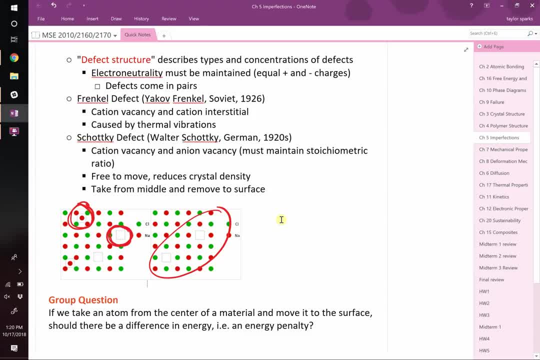 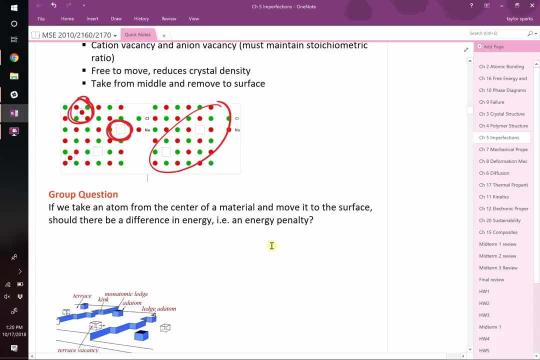 in electro neutrality. That's a problem. We're going to show you what happens in that case, right? First, let's ask this question: If we take an atom from the center of a material and I move it to the surface, is there an? 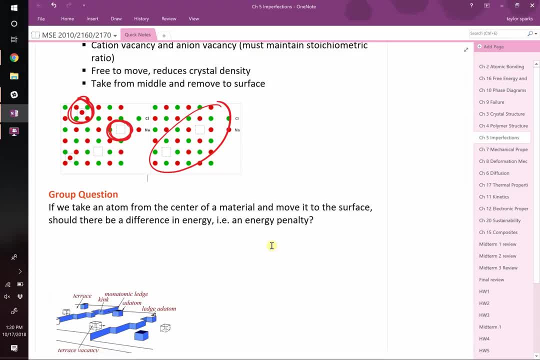 energy penalty. So imagine the students in this room If this block of students was totally filled and I pull a student out of the middle and I put a new chair on the surface, right on this front row here and I say: come, sit right. 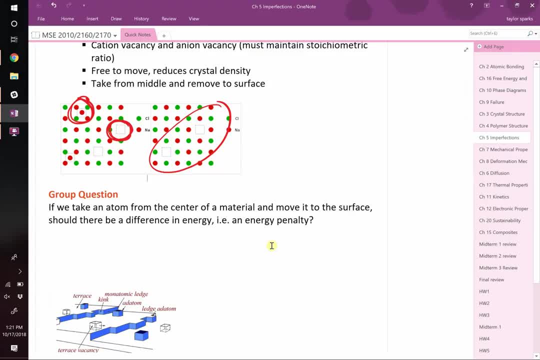 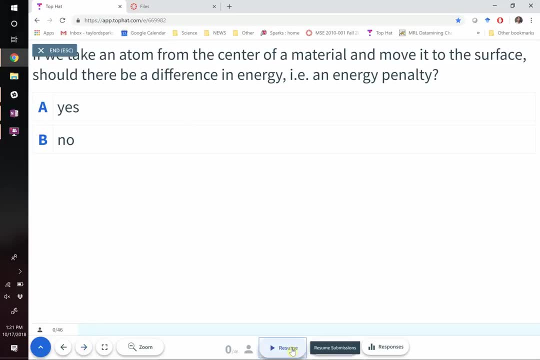 here. Is there any difference, Right, Yes or no? What do we think? I think yes. I think this is our next question. Okay, Is there an energy penalty, Yay or nay? If you pull it out of the center and you have it migrate to the surface, is there a penalty? 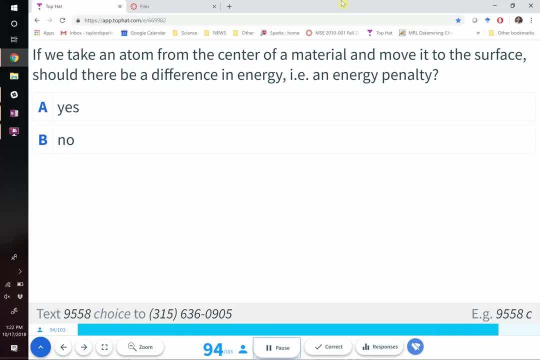 We pay for that. Okay, Get your answers in. We're going to close poll. Okay, What do we think? Yay or nay to an energy penalty? People think again, always 80-20, basically of people that get it right and wrong. 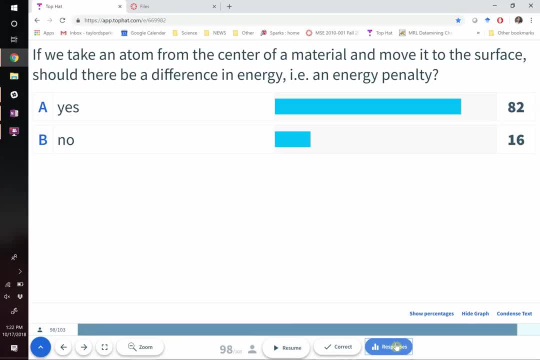 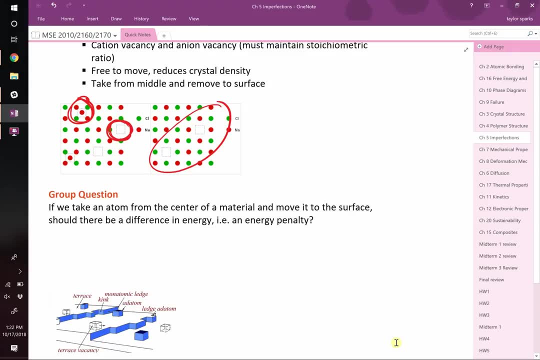 Yeah, It's an energy penalty Right Now. why is there Right Or an energy difference? For one thing, we've increased the disorder, Right, For sure we've increased the disorder, So entropy, that's going to change it. 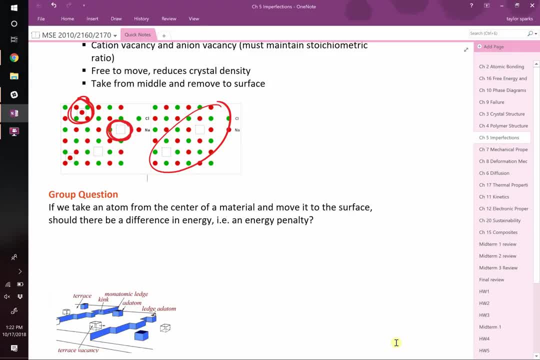 But also if we pull out somebody in the middle and they have like four bonds around them and we move them to a surface. now maybe it's only bonded to Hector Right. It's only got one bond and it wants to have four bonds. 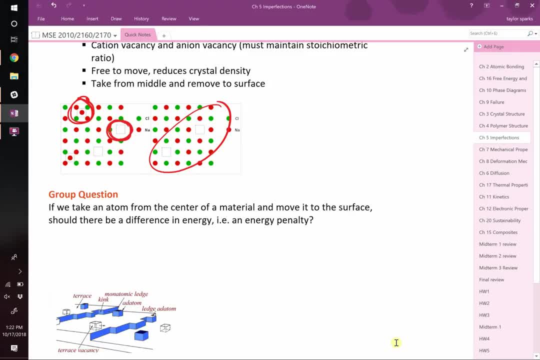 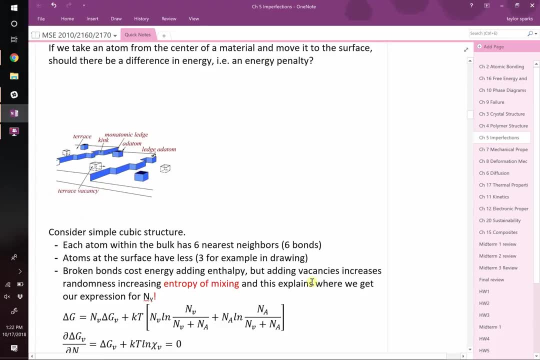 So we broke four bonds, We only made one. So there is definitely a difference in energy when you move something from the center of the material to the edge Right, And then it depends like, well, where does it sit on the surface? 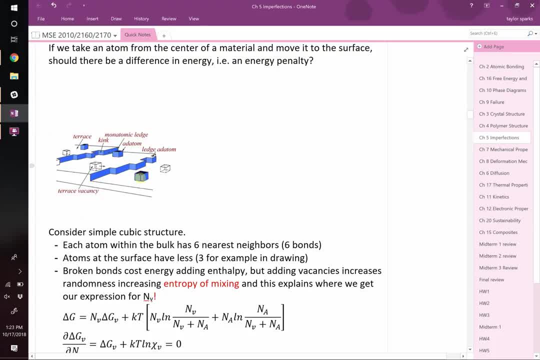 Right, Because you can have a blank slate where it just sits right here in the middle of nowhere. That has some energy. But what if there's a ledge of atoms and it sits next or on that ledge? What if there's a kink in that ledge and it fits in that kink? 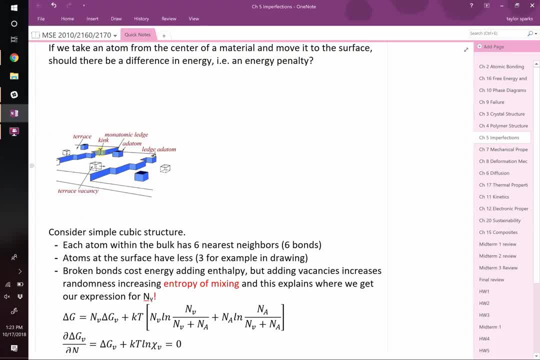 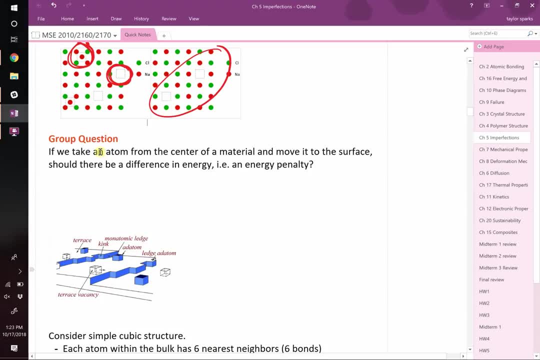 Each one of those scenarios is going to make a different number of bonds Right. This one sitting right here is going to have like one bond below it, This one that sits here, the next one that goes there will have one, two, three, the. 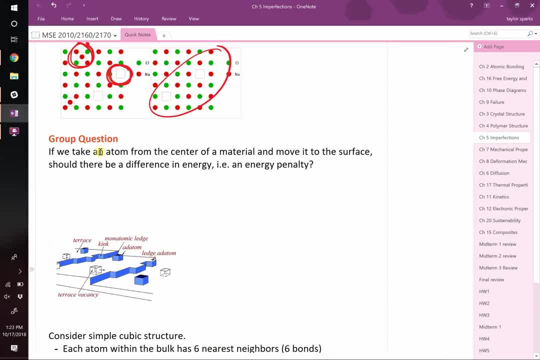 one below it Right In that kink it'll be maybe four. Right, There's different energies for sitting in different spots and because of that, when atoms do sort of grow on the surface of a material, let's say that you were sputtering. 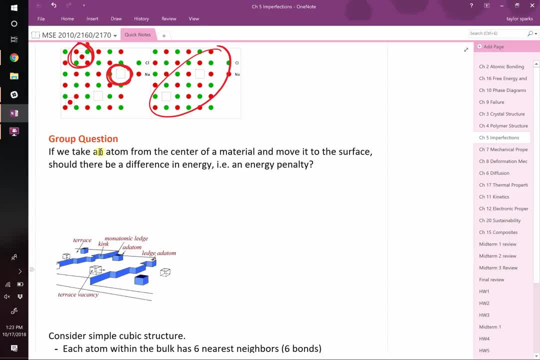 this with atoms, which is something they can do. They basically, from the gas phase, they bombard this with atoms. They then get to choose where they sit. They can choose to sit right here in the middle of nowhere, but that costs more energy. 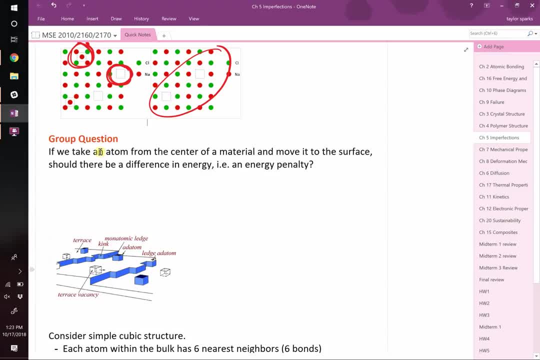 So instead they basically fill up these rows first and they sort of grow outwards and then it goes and it starts a new one. And you can see this because we live in the future. We have microscopes that let us see That. let us see atoms doing this. 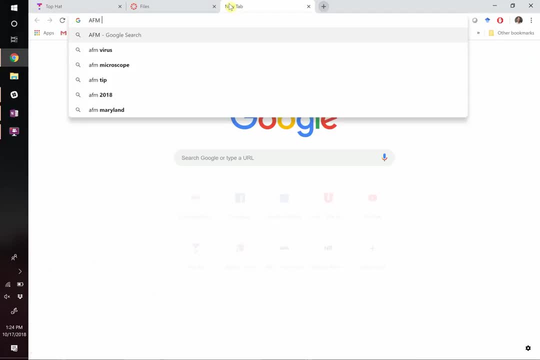 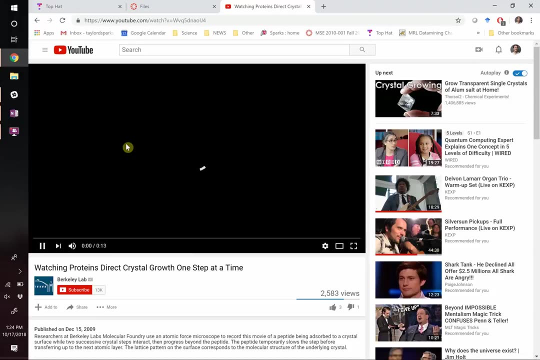 Should we do it? Let's do it. This feels right. AFM video: step growth. Let's see if that pulls it up. All right, Hopefully YouTube doesn't let us down. Yeah, you see that. See how they're growing from one side to the other. 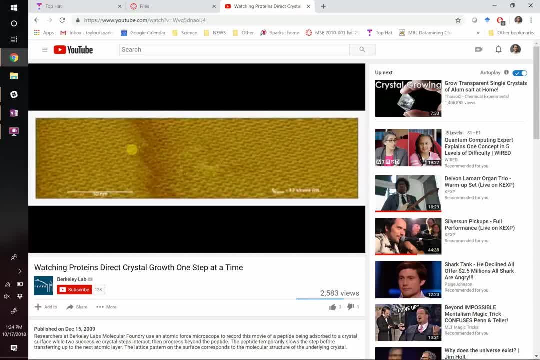 We'll see another one come. It happened quickly. Here's another one. See that How it's propagating. So this is an AFM image. AFM- at the end of this chapter we'll talk about microscopes. We'll talk about microscopes. 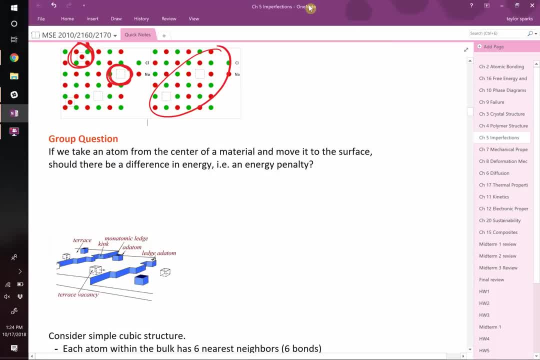 We'll talk about microscopes. We'll talk about microscopy techniques. AFM is one of them. It basically- I'll get to it later- It's a video that shows the surface. I'll tell you how it works at the end of this chapter. 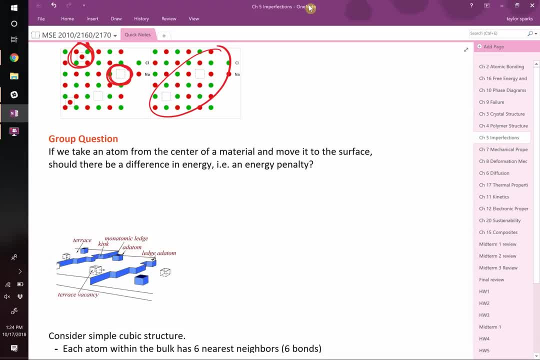 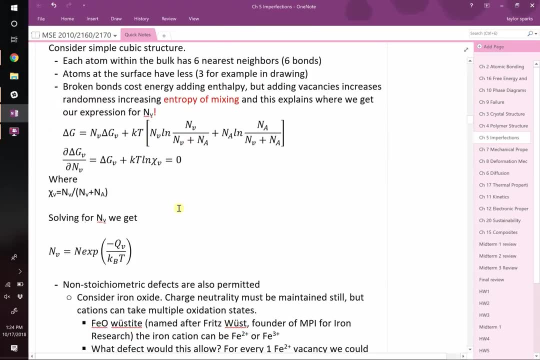 I'm not going to get out of order, But you can sort of see that happen because there's an energy difference on where these things sit. Okay, We're going to skip this math for the sake of time. Sorry, math. It basically just describes where this comes from. 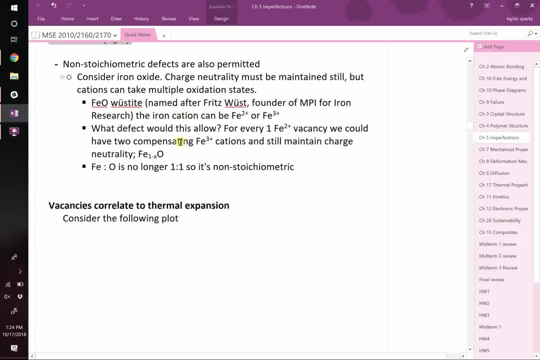 So if you want to know, it's there. Okay, Now when we dope things right, What happens when we dope things Or We've got these non-stoichiometric compounds? We've been talking about this a couple times over the semester. 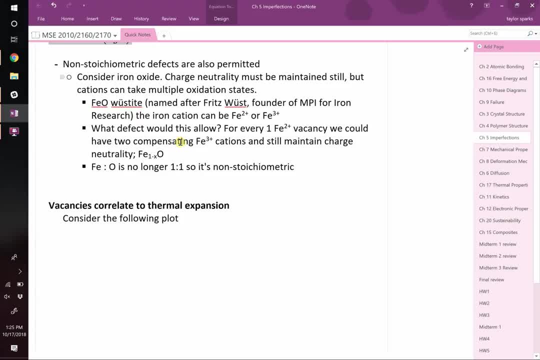 Our old friend Wustite FEO. we said Wustite is a problem because it gives us both Fe2 plus and Fe3 plus. By the way, this is named after the founder of the MPI. That's like Germany's version of the National Labs. 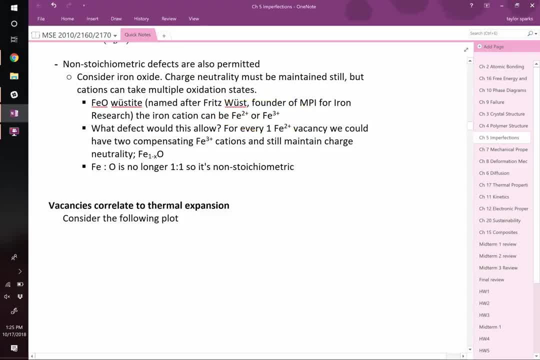 That was this guy. So Fritz Wust, I don't mind naming a chemical after you. That's a pretty good deal. Alright, So you've got these two different oxidation states, but oxygen is always 2 minus. So if you have pure Fe2 plus, then it's going to be a 1 to 1 compound. but we've talked. 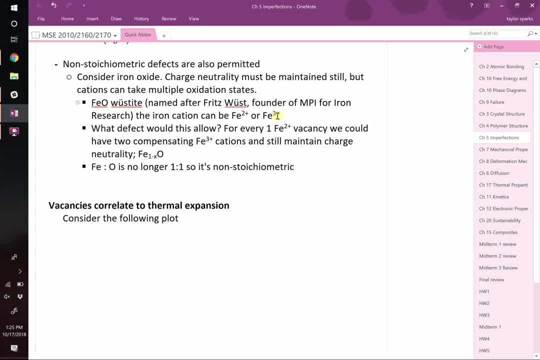 about. if it's both of those, it's going to be something other than 1 to 1.. You can have a non-stoichiometric compound, right? So that would be a different type of defect. that conforms right, Because in that case the vacancy on the iron site is compensated by the number of Fe2 plus. 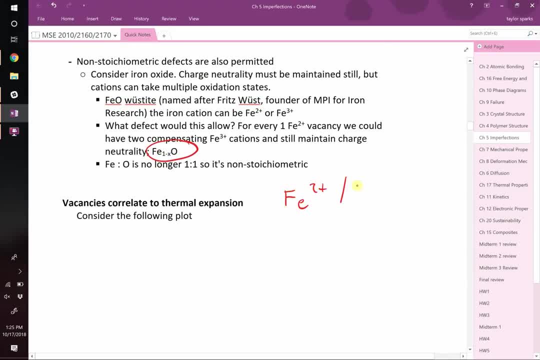 to Fe3 plus. right, You've got Fe2 plus and you've got Fe3 plus ions, Okay, And depending on that ratio, you will create iron vacancies. They'll call these cation vacancies as opposed to anion vacancies, okay. 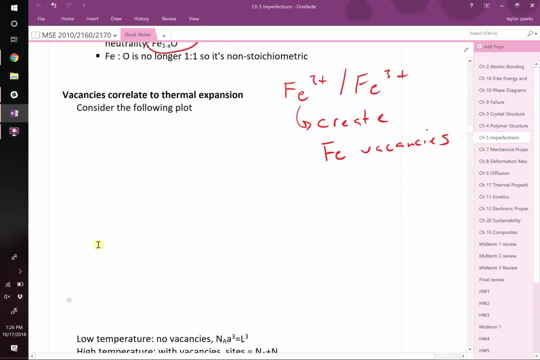 Now, something that's really interesting is that vacancies, even though there's not very many of them, they can influence properties. We already said they can influence electrical properties. They can also influence things like thermal expansion, and here's how. Alright, Let's look at the following plot. 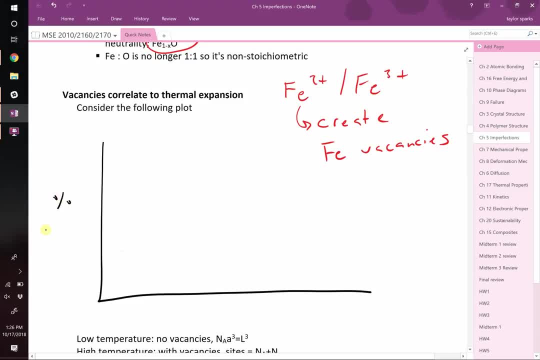 Let's say that you could plot percent change as you heat something up, So going to high temperatures. So I'm going to show two curves. First off, is your overall curve right? This guy right here, this would be delta L over L, right? 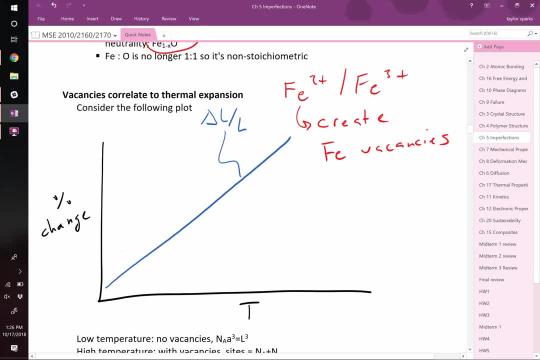 That's L final minus L initial, divided by L initial. Okay, Okay, Okay, Okay, Okay. So if you heat something up, it's going to expand and it let's say that it's a linear material. They don't have to be linear, but this one let's assume it's linear, right? 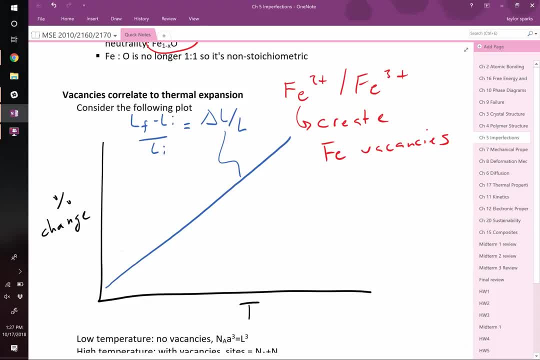 So it starts out, it's zero and it goes up There's. part of that is due to what we've already talked about in this class, which was what? What causes thermal expansion? Think way back to the very first chapter, to our old friend, the potential energy. well, 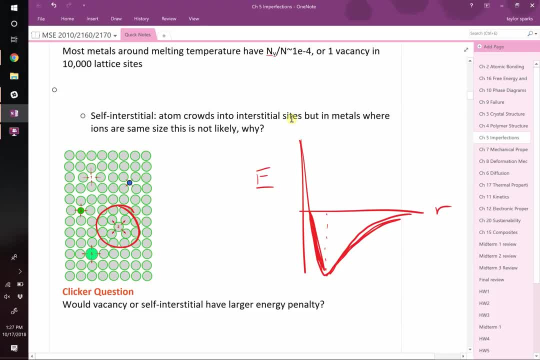 There's a reason. we covered this first, because it just keeps coming back. When you heat something up, you're giving it energy And the average position is no longer right here. right, The average position between here and this energy is maybe located slightly over and. 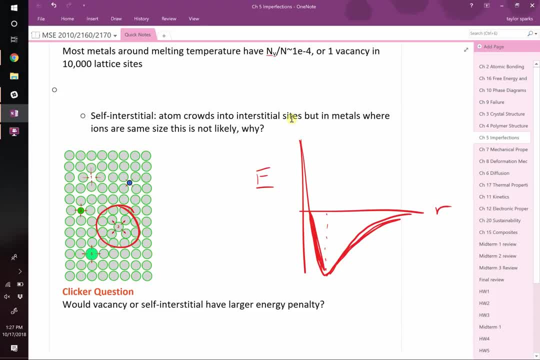 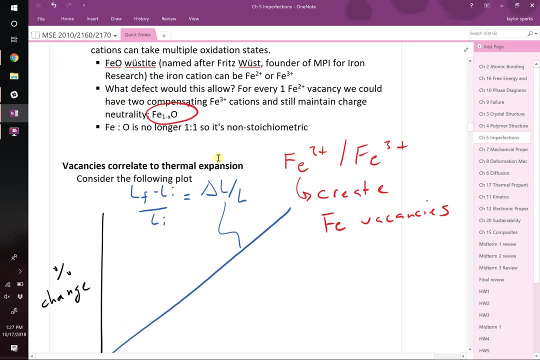 so it's expanding right. So the interatomic distances, the bond distances, are getting a little bit longer and, in other words, another way to say this is that the lattice parameter is increasing. okay, So if we were to draw a line that represents the lattice parameter change, it might do. 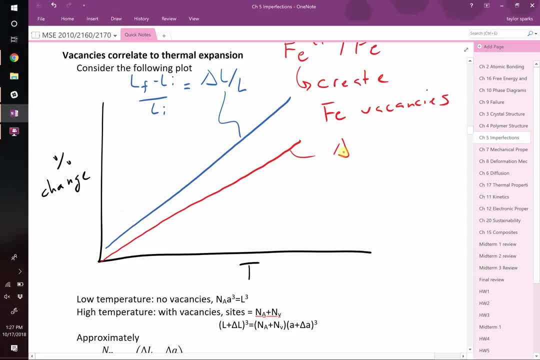 something like that. right, This would be delta A over A. Okay, So this is A final minus A initial divided by A initial. okay, That's our lattice parameter. So the key thing I'm telling you here is that lattice parameter alone can't explain the 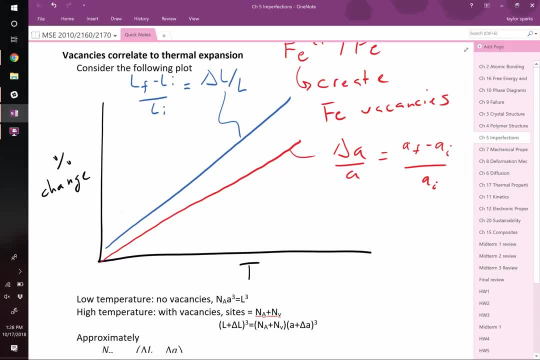 total change in length. There's an extra amount, right, And that's coming from vacancies. This is shocking. Think about what I'm telling you. If this room was totally packed, let's imagine all these students crammed into the smallest number of seats possible, and then I heat them up, right. 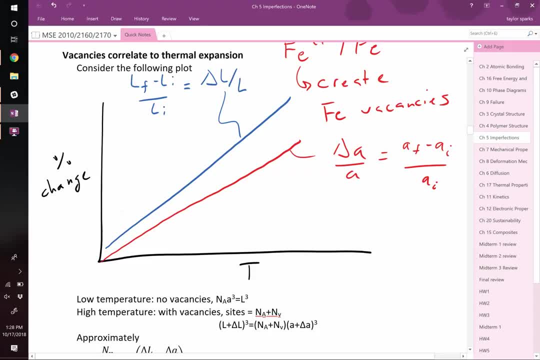 And they're hot so they want to get away from their neighbors. So they start spreading out a little bit. It's going to expand a little bit, but in addition, the people in the very middle, some of them, a small fraction of them anyways- are going to get up and say I'm sick of this. 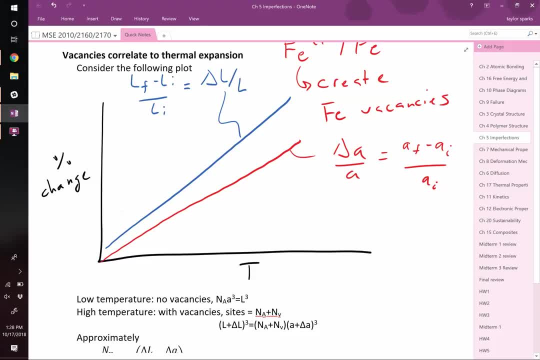 middle business. I'm going to move to the surface right, And if enough of them do that, by moving to the surface, you made the overall thing a little bit bigger right, And it's big enough. you can actually see it with measurements, right. 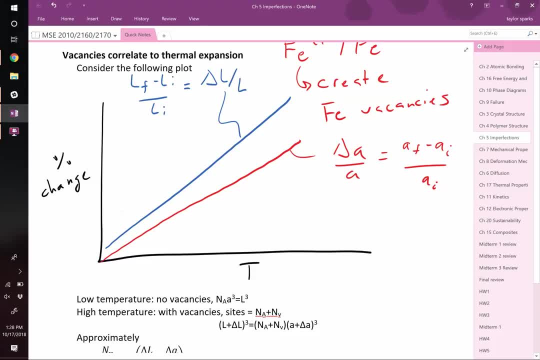 You just don't look shocked. That's shocking right. We're talking like one in 10,000 atoms is your vacancies and yet it's enough to make significant right, Significant changes on like. if you have like a ruler on a material, you can see it. 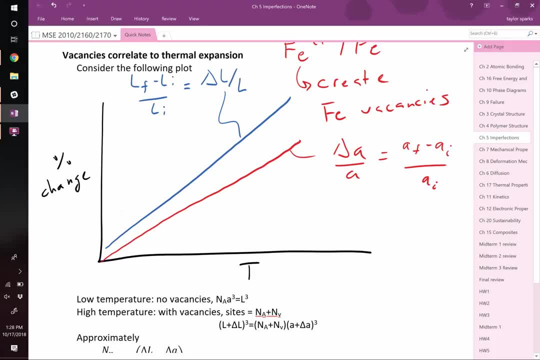 getting bigger, and a fraction of that comes from vacancies, right? So this difference here between the two curves, this difference right there, at any given temperature, the difference that's going to be equal to NV divided by N, divided by three, right? 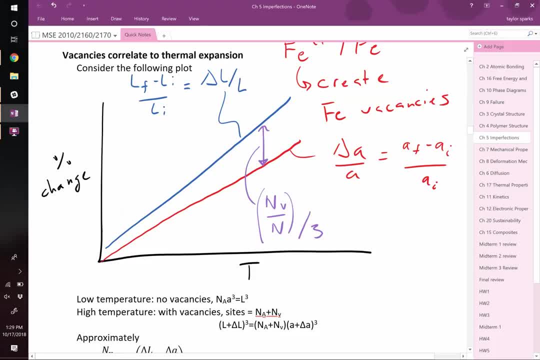 It's our vacancy concentration divided by three. Okay, Yeah, question Sam. I'm just wondering if you could talk about how the vacancy can happen. I guess, because they just like Great question, How would it happen? So, if it's like way deeper than the middle of the material, how did that thing get all? 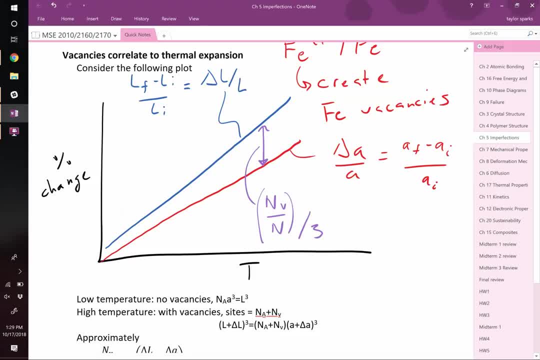 the way to the surface. It's a hopping mechanism, okay? So let's say that there's an empty seat right, Right here we've got an empty seat right. So if we, if, if- don't tell me it starts with an A- hardly, hardly. 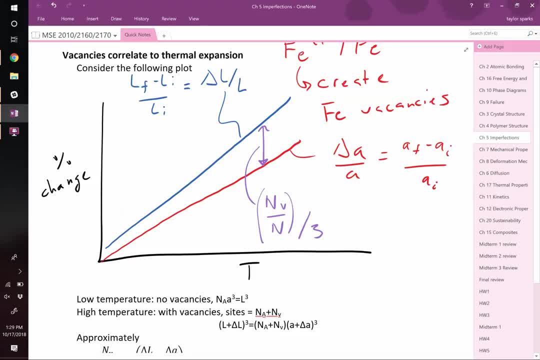 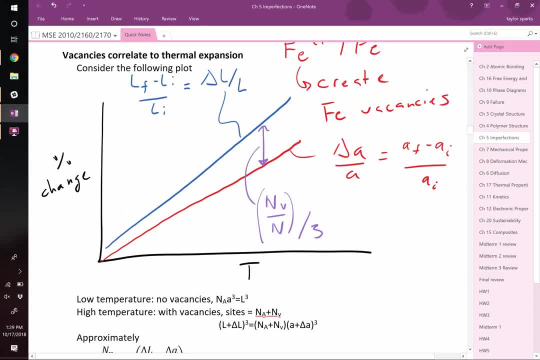 He's going to get to the front. What really happens is like it's a series. So all atoms are indistinguishable, right? So that exact atom doesn't have to get to the front. We just need an empty spot there. So if I was sitting here, right? 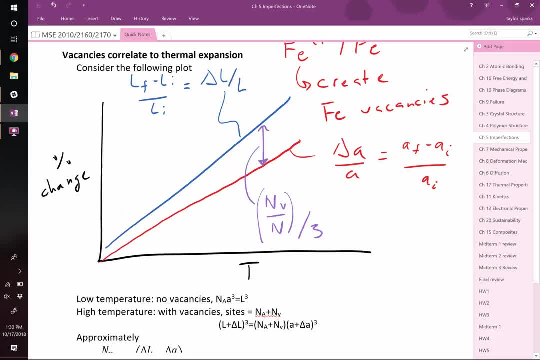 There's the empty seat here. I could hop to here, and now there's an empty seat. Somebody else like hardly could hop to there. the empty seat right Next thing you know, the vacancy is all the way in the middle. 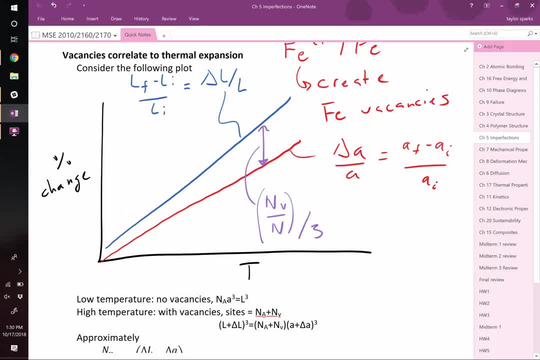 So it hops from the surface inward. That's kind of how it works. okay, There's other ways it can happen. It can go along grain boundaries. We're going to talk about this in the next chapter in diffusion right. This is the lattice where everything's sort of ordered. 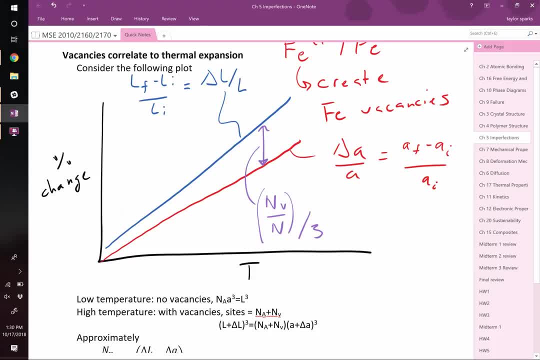 But what about this region in between? So if I have the choice to move through the material, I could try and like climb over people, but that's going to strain them and cost energy. We're going to like walk down the aisle right. 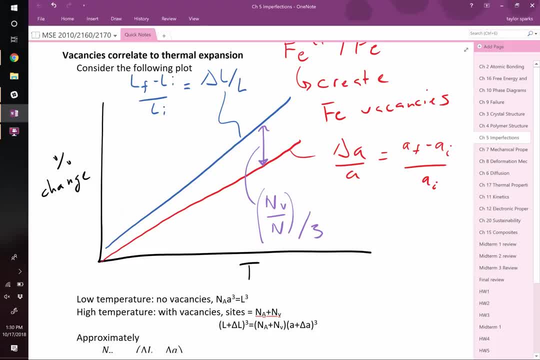 So, like grain boundaries are diffusion short-circuit pathways, Things can move much quicker along grain boundaries and other things which we'll talk about later. Okay, any other questions on this? On how thermal expansion is the blue? That's what you measure, right? 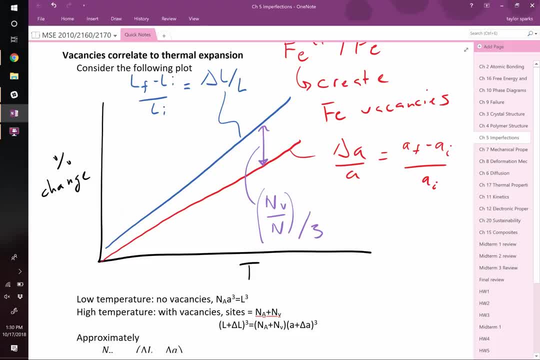 If you had like a ruler or calipers and you measured the length of something as you heat it up, you're measuring the blue line. X-ray diffraction or other tools can give you the red line and I'm telling you that there's a difference between that. 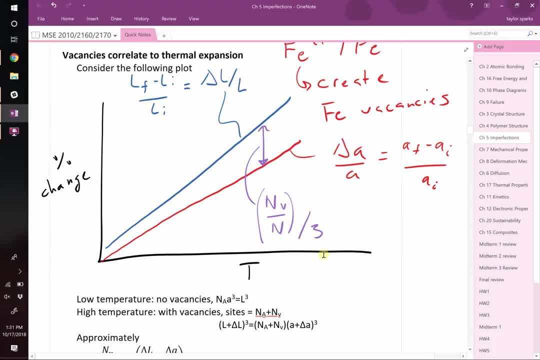 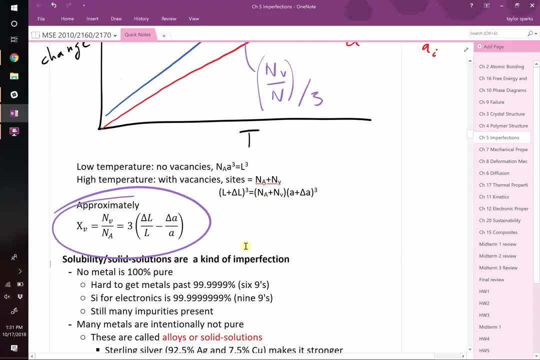 and that difference is the vacancy concentration. okay, So there's an expression on the homework. you're going to use this, So hang on to that in your back pocket. There's a homework question on it. Okay, we've talked about pure metals versus now doped materials. 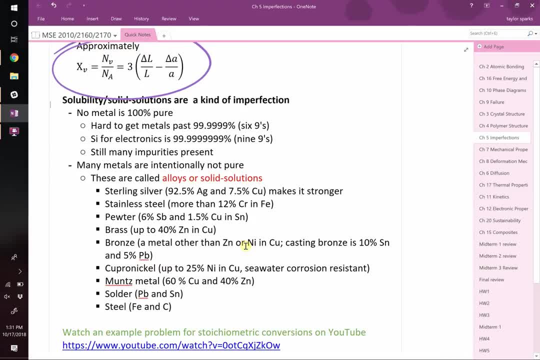 We've said that. you know, oftentimes pure metals or materials aren't even what we want. Sometimes they are right. If you're making integrated circuits for computers and things like that, they want incredibly pure silicon. In fact, you might not know this, but like places like Intel and them. 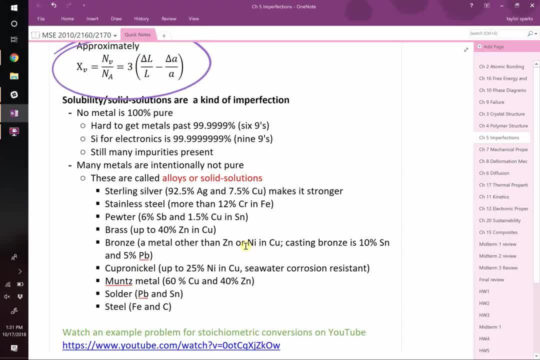 what does silicon come from? It comes from sand. They start from SiO2, and they don't even get it from just anywhere They buy it from like specific sand dunes in the world that are like high, high, high purity. 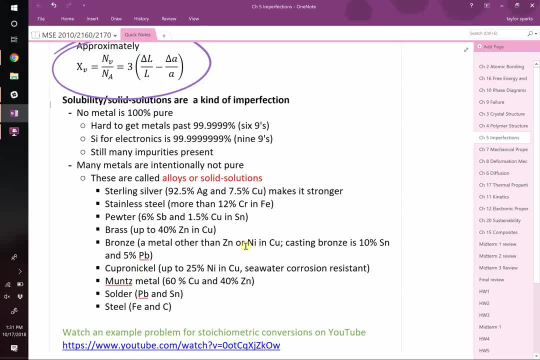 because it's just too hard to refine out. so they actually get their quartz not from like Long Beach but from like specific spots in the world with high purity sand, and they can get it to what's called 9-9 purity. 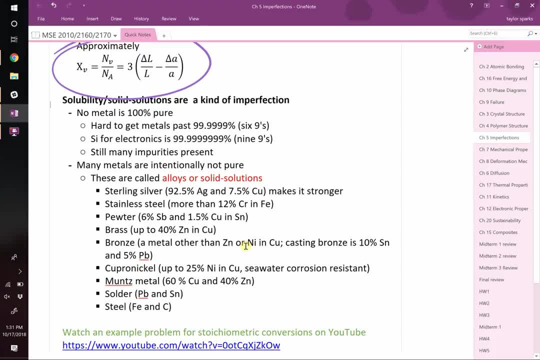 That means it's 99.999999 and so forth until you have 9-9s purity. What that means is: I used to have it. I think that's like one in a billion atoms are not silicon, so incredibly, incredibly pure okay. 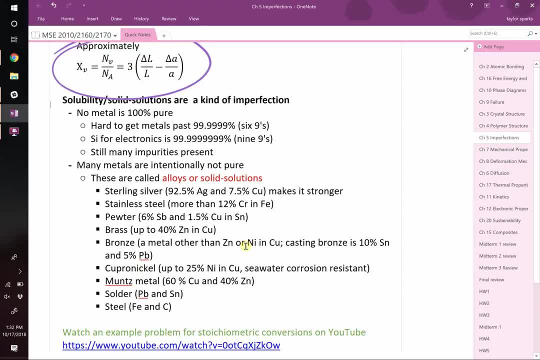 Um, It's very hard to do that. It's hard to even get what's called 6-9, and you pay for it If you guys go out and work in industry and you naively think, oh, my boss wants me to make whatever compound. 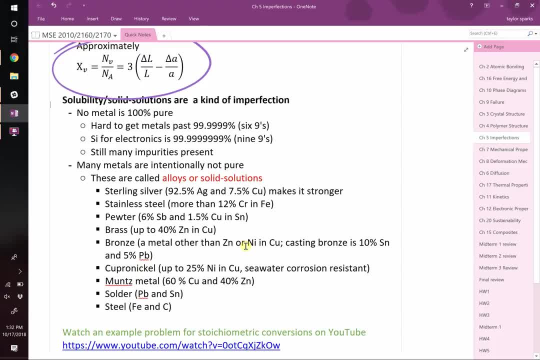 I'm just gonna order really pure materials because that seems like the thing to do. they cost crazy amounts of money right 5- or 6-9 purity, like Logan. what does it cost to buy that, To buy even cheap stuff like iron at 9-9 purity? 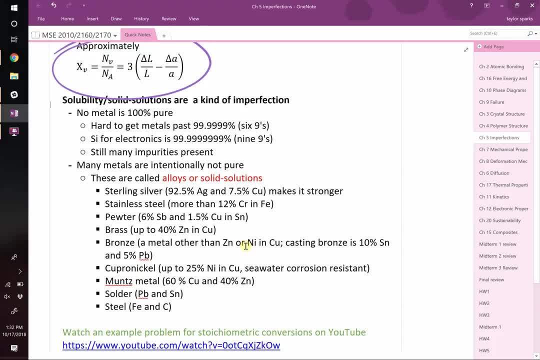 will cost you a couple hundred bucks for maybe 100 grams, right, Very expensive. And if it's a And that's for a common material, Then if you want ultra-pure something like scandium, right, Which is rare to start with, forget it. 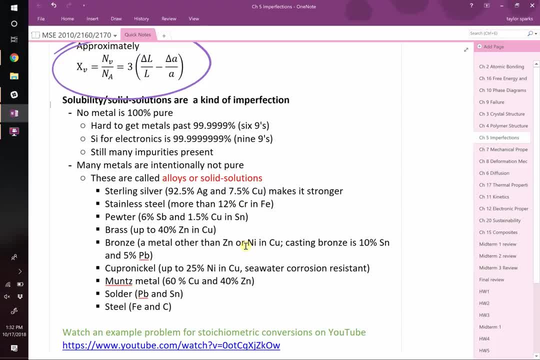 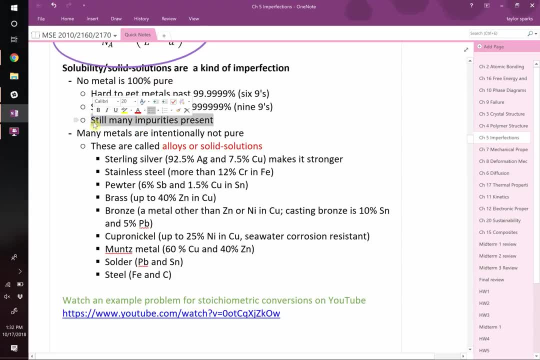 It's just crazy expensive. So that's purity. We don't have time to talk about how you purify things, but impurities often get left over, and sometimes they get left over by design, right. So alloys are things where it's left over by design. 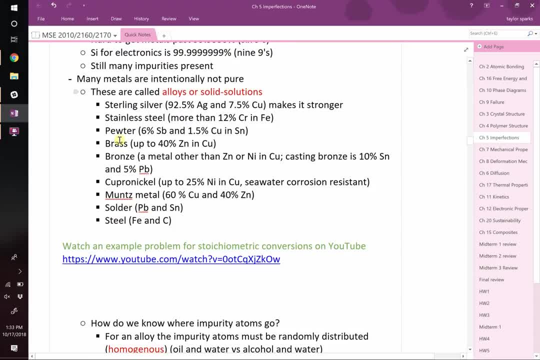 Sterling silver. you've heard of sterling silver. That is 92% silver and then it's. the rest is copper. The reason they do that, for one thing, copper's cheaper right. But the real reason they do it is because adding copper 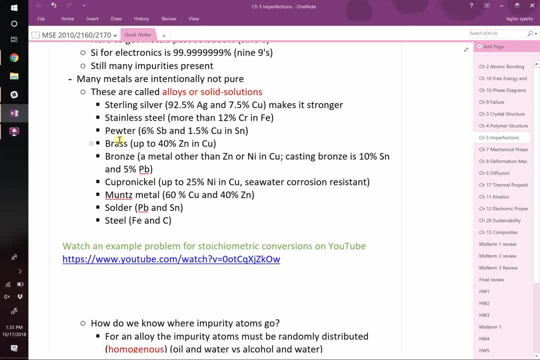 changes the properties that you care about, namely the hardness and the yield strength. It makes it more scratch-resistant- and we will talk about why in a few chapters- But adding a little bit of copper, even though it's a substitutional alloy. 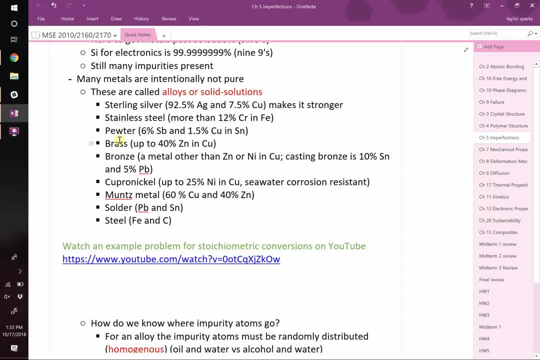 it substitutes for silver, it makes it harder and therefore it's scratch-resistant, which you want if you're going to make it jewelry, okay. But there's stainless steel. we've already talked about that. You take out some of the iron, you put in at least 12% chromium. 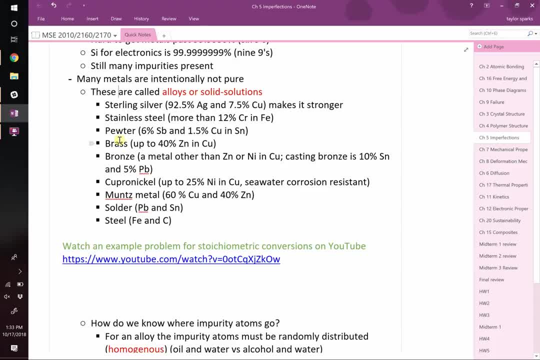 Now you've got this nice oxide layer that forms because the chromium is there, Because the chromium oxidizes and protects it. You've got pewter, brass, bronze. all these things are mixtures. They're intentional mixtures of metals that have some exact property, like muntz metal. 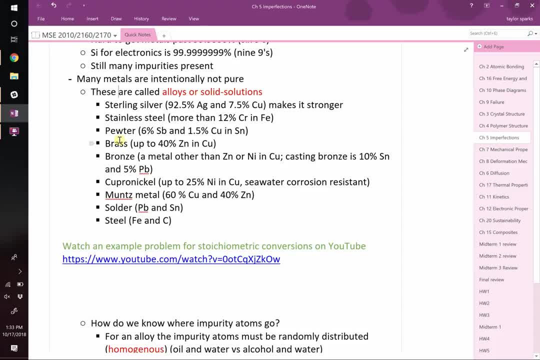 They use this to make it's corrosion-resistant in salt water, right, Just like the one above it. Both of those things are pretty corrosion-resistant in salt water Solder we've talked about, So there's lots and lots of alloys that. 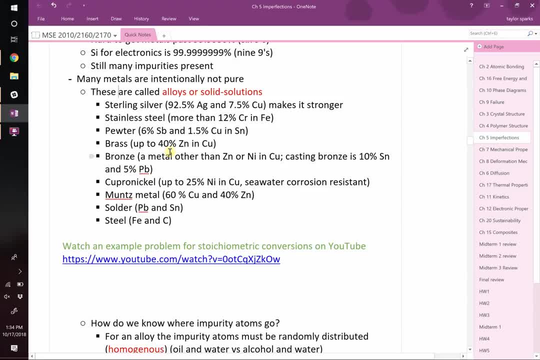 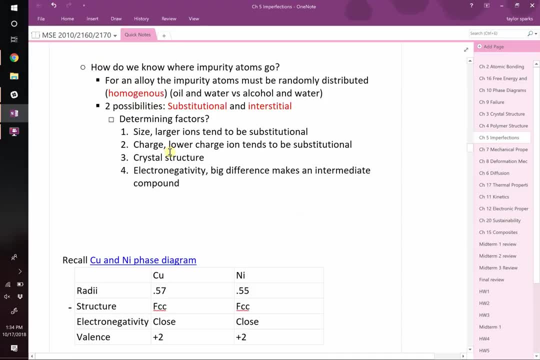 you should be aware of that. they're not pure elements, but they're intentionally solid solutions, okay. Okay, how do you know where an atom's going to go? We've already said that. if I've got a doping atom, if, let's say, all the students in this room are copper, 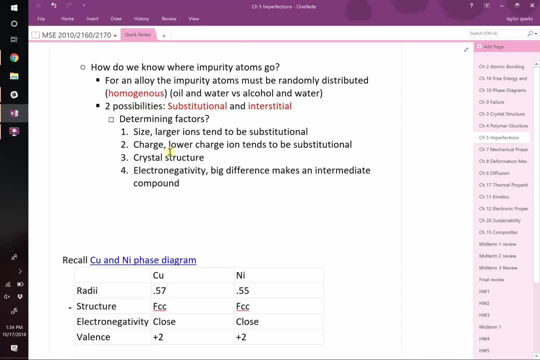 and I've got a nickel atom and I say, you know, I'm going to mix it in with that. where's it going to go? Is it going to ask Elias to get up and move and sit somewhere else and take his seat? 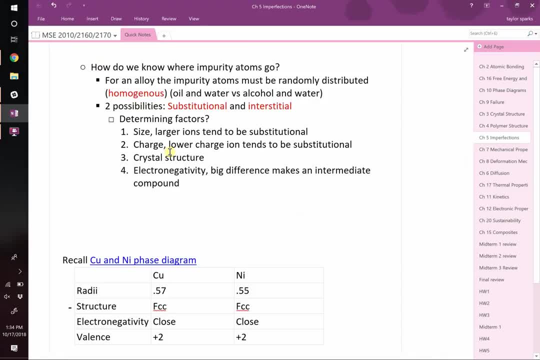 which is a possibility. That's a substitution, a substitutional thing, Or is it going to be interstitial right? If he sits next to our sleeping friend here, then that's an interstitial right. He's like going to be crowding and he's awake. 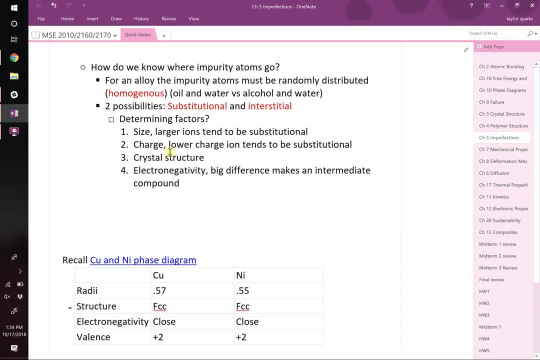 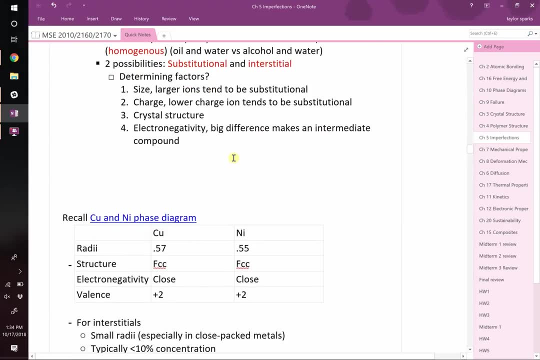 Right. So you have the option: substitution or interstitial. How do you know which one it's going to be? So there's some general rules. Here's our rules. If it's the same size, it's more likely to substitute. 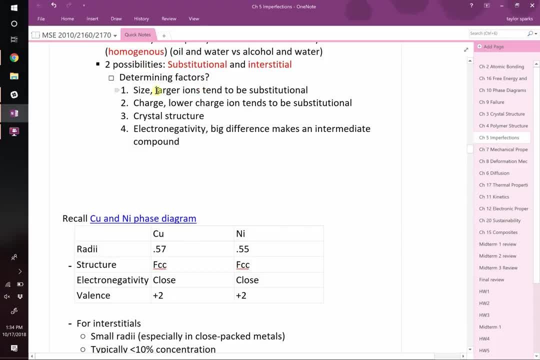 If one is larger than the other, sorry, the larger ion will substitute, right? So again, let's say: you've got like the Kool-Aid man and the Kool-Aid man wants to take a seat if he tries to sit in an interstitial. 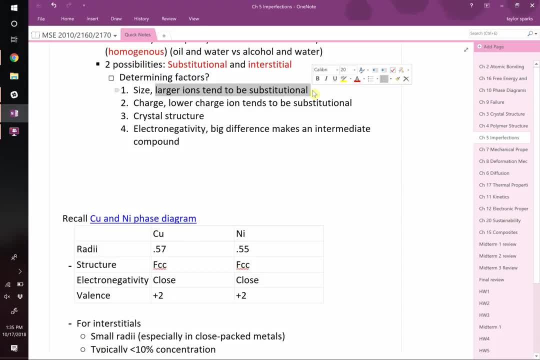 that's not going to work. He's more likely to kick someone out of their seat. right Charge. lower charge ions tend to be substitutional. That's really the same reason as before. Lower charge ions are bigger ions, so they tend to substitute. 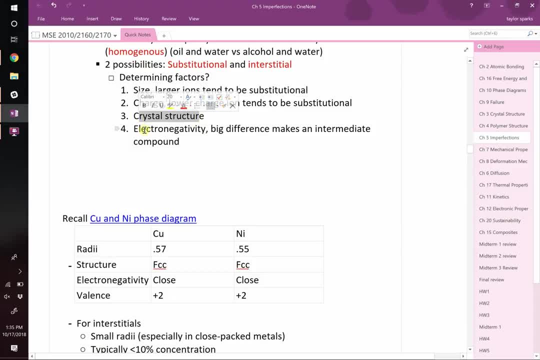 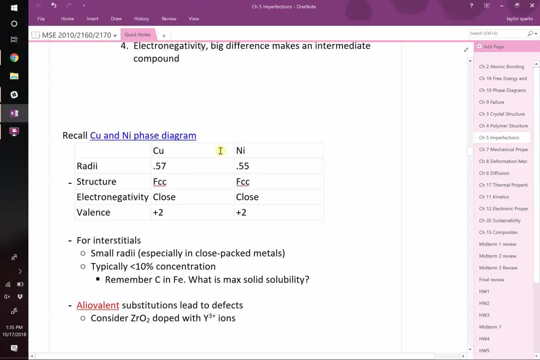 We get substitution if you get the same crystal structure and if there's not a big difference in electronegativity. If it's not the case for any of those four rules, then you're likely to get interstitial. Alright, let's get to the 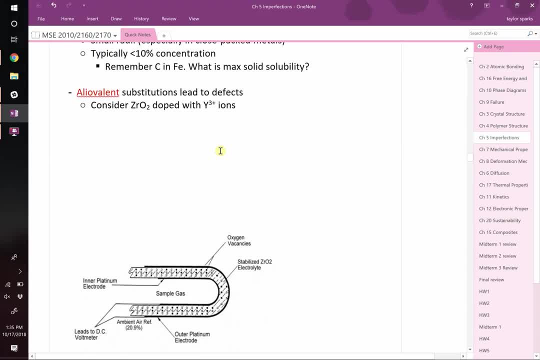 most interesting thing when it comes to these dopants: What do we do with a different charge? right, Let's take yttrium 3+? right, That's our ion and we're going to substitute it in to zirconia. 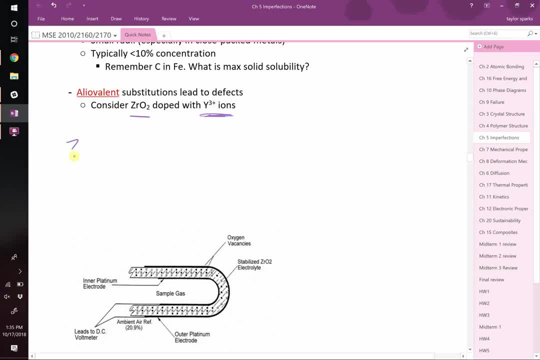 right. Zirconia, ZrO2, in that structure it's Zr4+ right Because there's two oxygens. so you have to have four positive charge to have this thing balance out. So what happens if I pull a zirconium out? 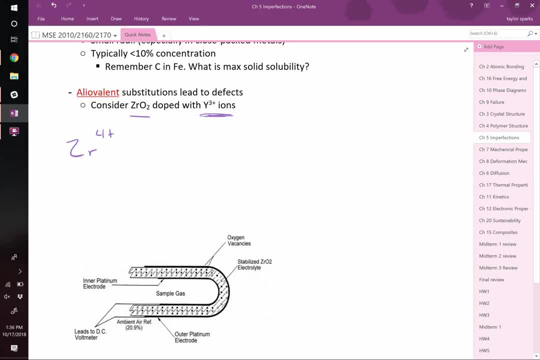 and I put an yttrium in. it's not balanced. That neutrality has to be conserved. So what will happen? Maybe turn to a neighbor? What will happen if we put in an yttrium on a zirconium site? 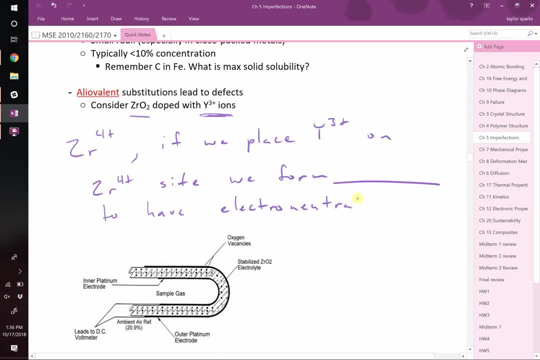 And the picture kind of gives it away. right, You're going to have oxygen vacancies, right? So by putting in a 3+ on a 4+ site you don't have enough positive charge. So you can either try and add extra. 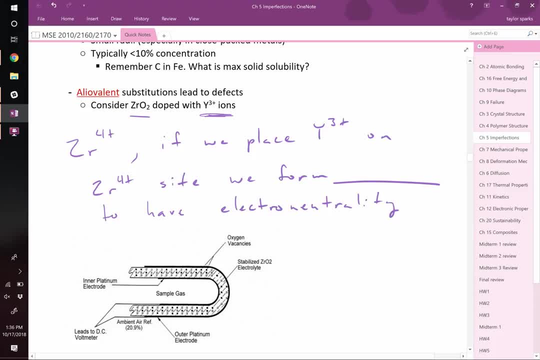 positive charge, but that's going to mean putting extra yttrium in interstitial spots. Interstitial spots cost a lot of energy, right? So you're cramming extra atoms in. That's less likely. The other option you have is forming oxygen vacancies. 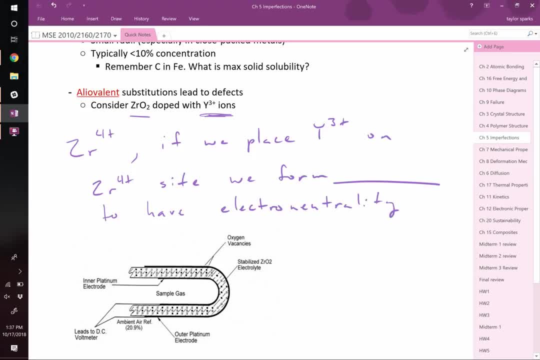 because if you take out an oxygen, they have a negative charge. So you could, by having this yttrium, which doesn't make it positive enough, if you pull out some of your negative, you can make it work. So how many do you have? 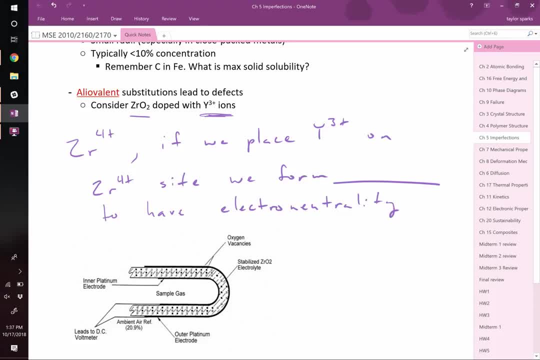 For every one yttrium substitution, you are deficient in your positive charge by one. 3+ on a 4+, you're deficient by one, But oxygens come in a charge of two. So what you have to have is for every. 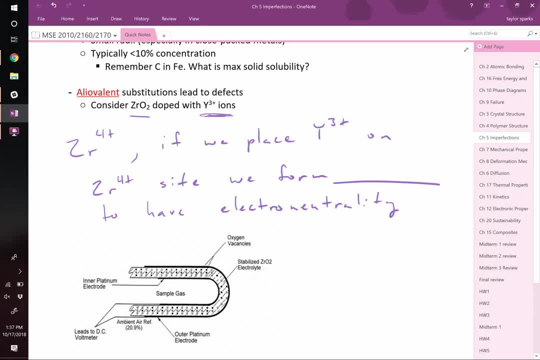 yttrium. for every two yttrium that you substitute, you have one oxygen vacancy. That make sense. Two yttriums. now you have built up a positive two that's missing, So you make up for that by pulling out a negative two ion. 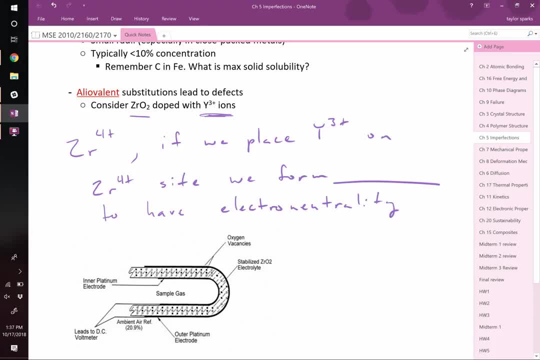 Make sense. Are there any questions? Yeah, So yeah, you can have. what do you call these co-doped samples? Co-doped samples is one's exactly what you're getting at: You dope one thing, but you also dope the other. and then you're left with no vacancies. afterwards It's going to depend system by system and dopant by dopant if that's more favorable than forming vacancies. It totally depends. In general vacancies don't cost that much, but interstitials putting something else on there. 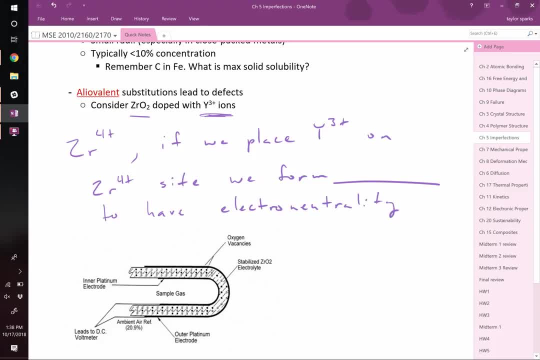 tend to cost a little bit more. They tend to be much less likely because the size of ions is rarely the same, and so there's usually crowding of some sort. So why do we care about this? So this is what happens. This is amazing, right. 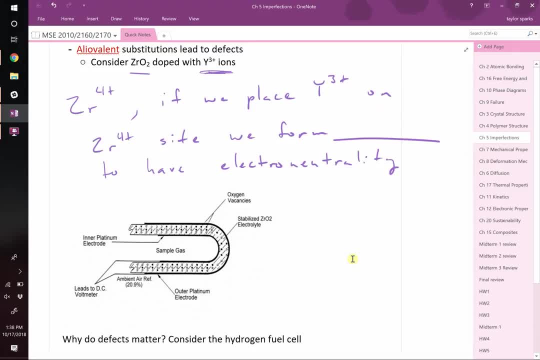 Remember the same zirconia. that was amazing because it's kind of like steel and that it's tough. Remember how that worked? We said that you doped it with something, You dope it with yttria, just like this, And what we said happened. there was that. 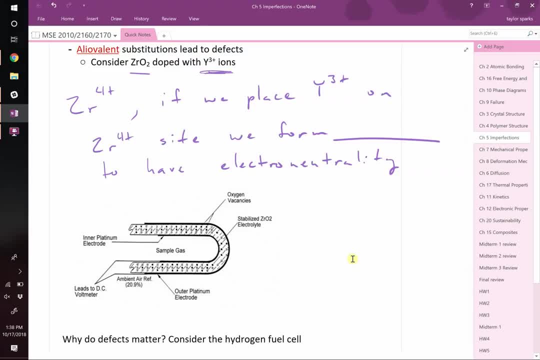 at high temperatures. there's a phase that is kept in a metastable state at room temperature and then, when a crack comes nearby, that phase expands and it closes the crack. So a completely unrelated phenomenon in the same material is this: Now we've got oxygen vacancies. 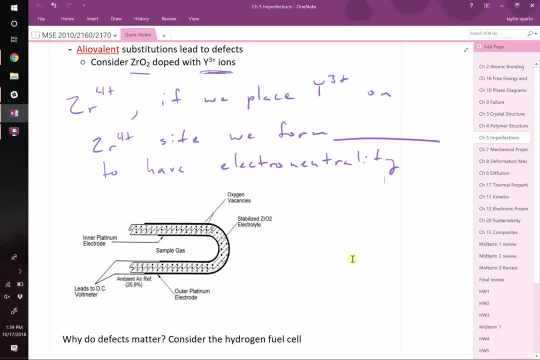 but it makes it incredibly important for a different reason. If you have oxygen vacancies, that's like having empty seats in this middle block of students. If there's empty seats and somebody wants to slowly hop their way to the back of the room, you have a pathway for that to happen. 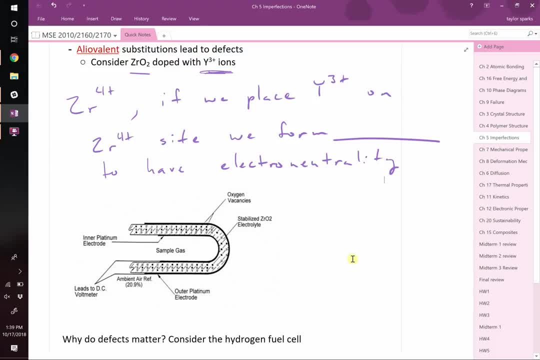 If every seat was filled, then you're climbing over people and that's not ideal. But if there's empty seats and you can hop, that's pretty good. So that's what happens here. You make sensors out of these, so this is in every single vehicle ever. 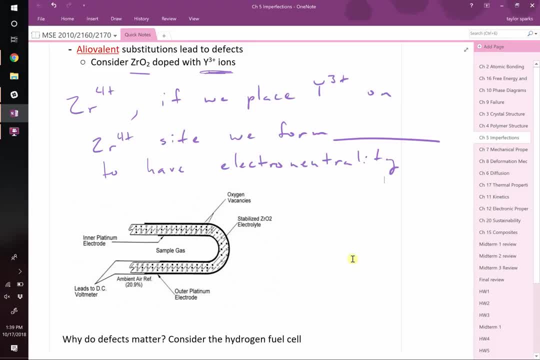 Well, new vehicles, Old vehicles didn't have it, But new vehicles all have fuel injection or they have at least an oxygen sensor. How it works is: you've got this sticking into your exhaust pipe, so you've got the effluent coming out of your motor. 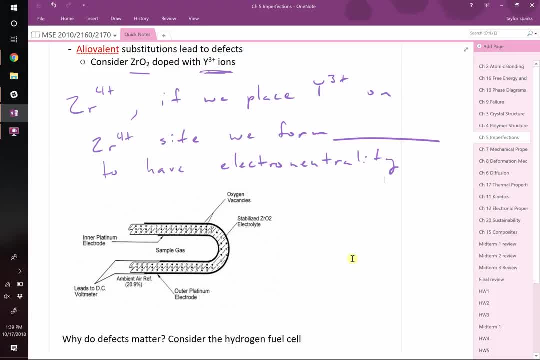 and if you've tuned your car motor correctly, then you have the precise ratio of oxygen to fuel, such that it burns, and you're not left with any excess unburnt fuel- soot. It's not good for anything, right? You want to burn all of that. 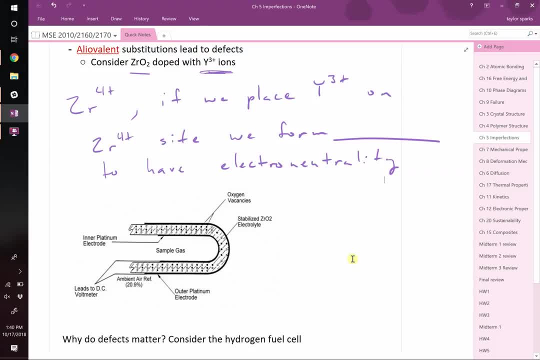 so you consume the correct ratio. but the problem is that ratio needs to be tuned as temperature and altitude and all these other conditions change slightly. so what you need is you need a way in real time to figure out how much. let's see which side's which. 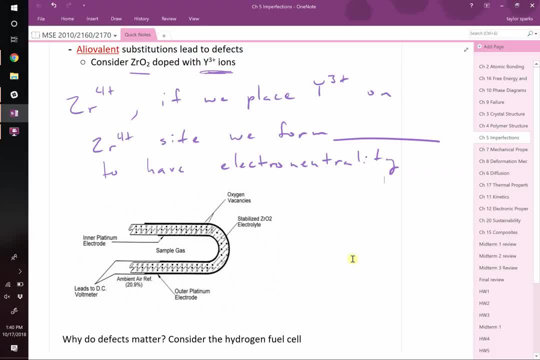 this is ambient air, this is sample gas. so inside your catalytic converter, inside your effluent gas, you need to figure out how much oxygen is there. If there's way too much oxygen, then you're not adding enough fuel. You don't have enough air to it, right? 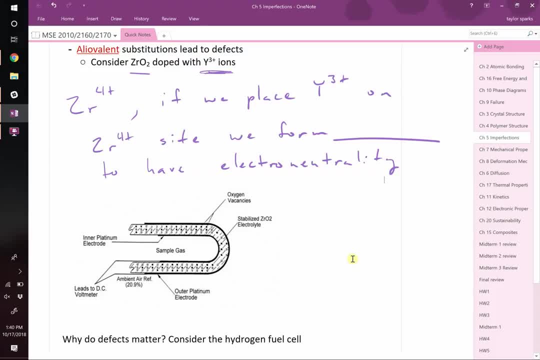 So you need to be able to tune that so they embed these things here, and how it works is amazing. in air you've got 21% oxygen, and if you have no oxygen, here there's a gradient in the concentration. therefore there's a driving force. we're going to learn about this next chapter.